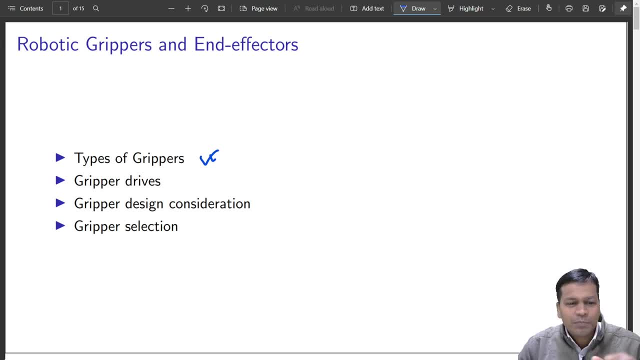 Which can hold something, which can pick a part from a place and it can put it to some other place Effectively. it can hold something Okay. it can hold something Okay, whether it places it or not. that is a different issue. There are many other types of end effector which are there Okay. other types of end effector include welding, welding gun, polishing gun. right, You can have a end effector that can do both. 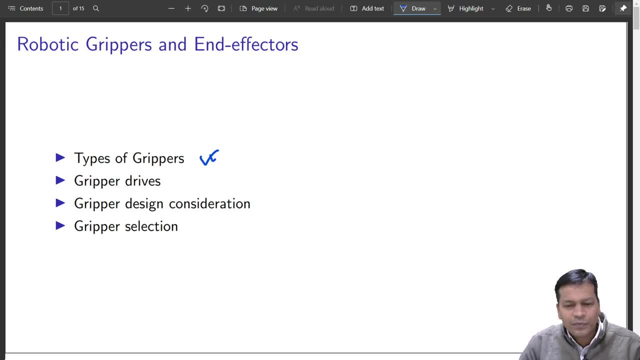 Grinding, also spot welding. So these are all different types of end effector. Gripper is one of them which can just hold an object. So we will specialize today's talk mostly on grippers. Okay, while doing so, we will talk about different types of gripper. gripper drives- Okay, what all types of drives that are there? What are different design considerations which has to be taken care of while designing a gripper for a project? 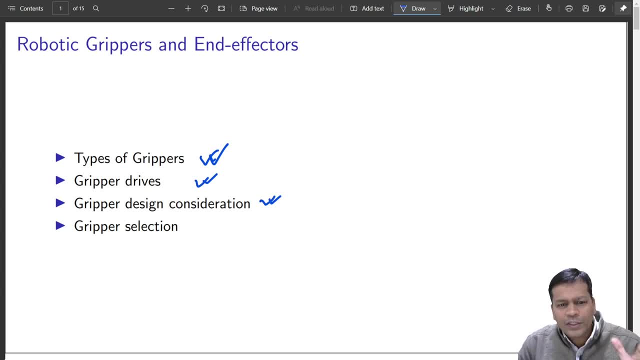 No particular application. or rather, let us say, you have a job in hand, you want to do that job. So what all gripper types, what all factors that you will consider while selecting a gripper from a given choices of gripper? okay, which are available in the market? Okay, so that is why it makes this very, very important. Okay, so at least one, something that can do some sort of end effector job. that is a gripper. 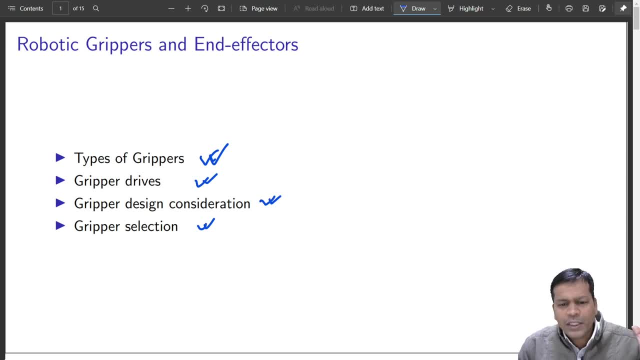 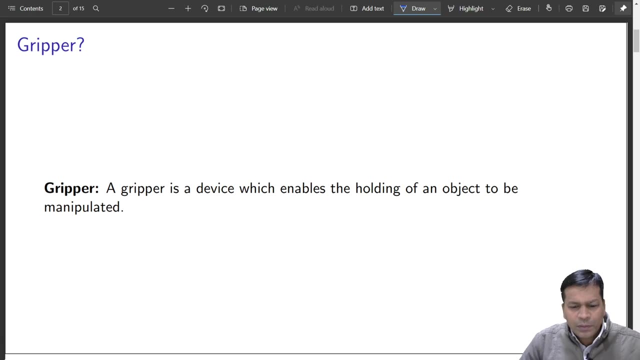 Gripper will do. Okay, we won't be doing any other type of end effectors in this course. Okay, so robotics, gripper. So let us begin down then. Okay, so effectively. as I have told you, gripper is a device that enables the holding of an object to be manipulated- Okay, manipulated- which can be taken from a place or put it to some other place. it is to be picked up or installed. 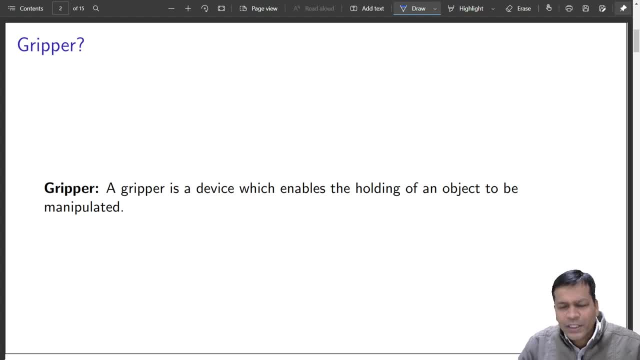 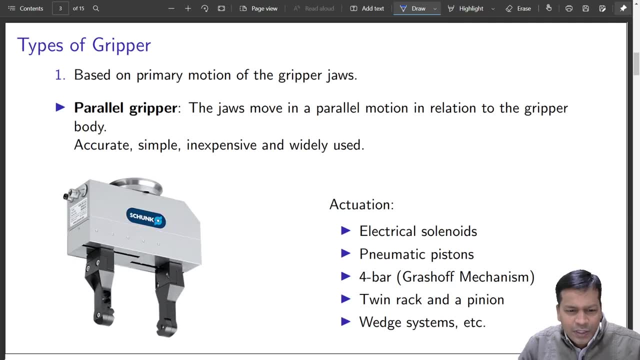 Okay, or you have to hold something and hammer it something, Okay, so that also is a gripper's job. Okay, so different types of gripper will first look at. look at different classification is what goes in classifying? classifying, given a type of gripper, Okay, we can bid classification. does it belong to what? all actuations, based on the way it operates, based on the actuator does it have? 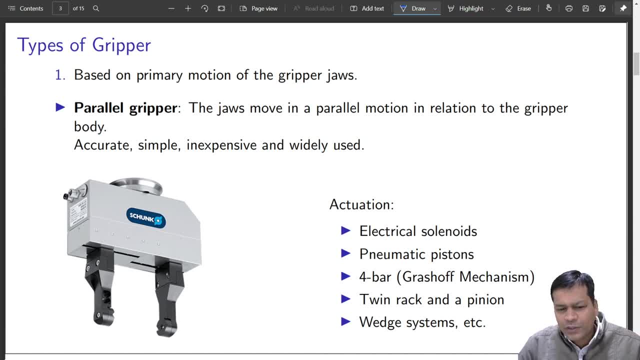 Alright, Okay, Alright, Great akh, Alright, Okay, Okay, Okay, Excellent. have, or based on the primary motion that a gripper jaws can do. so it can be done in various ways, so this is one of them. 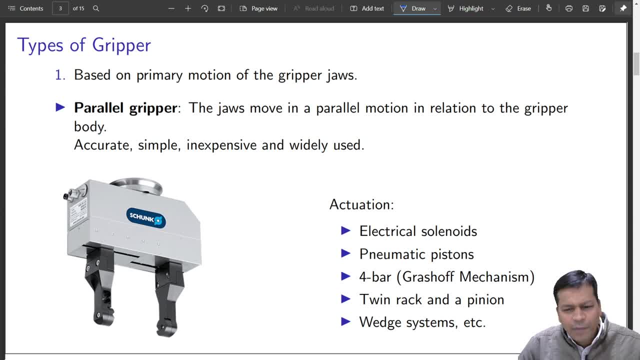 So we are classifying first using primary motion of the gripper jaws. primary motion of the gripper jaws. So what? the first one that shows is a parallel gripper, parallel gripper, In this case the jaws. the jaws move in parallel motion in relation to the gripper body. 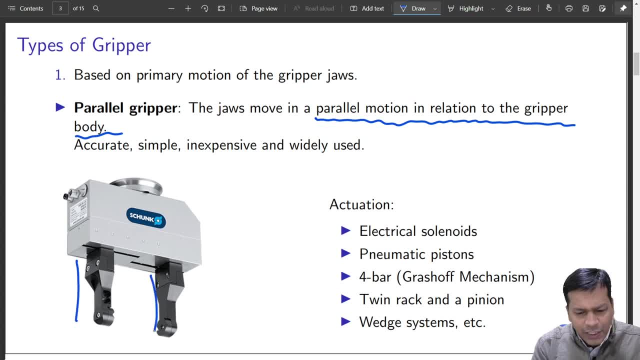 So, yes, there are two fingers that you can see. they will always remain parallel to each other and they can go closer and they can go wider. So that is something that it can do and it is always in line with this body. It will always move along this. 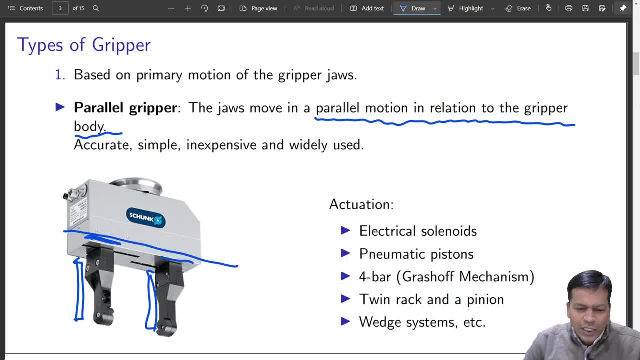 Parallel to the body of the gripper itself. So that is the direction of motion. these two are direction of motion and they always remain parallel to each other, So that is why it is known as a parallel gripper. This type of gripper is very, very accurate, very, very accurate, because there is hardly 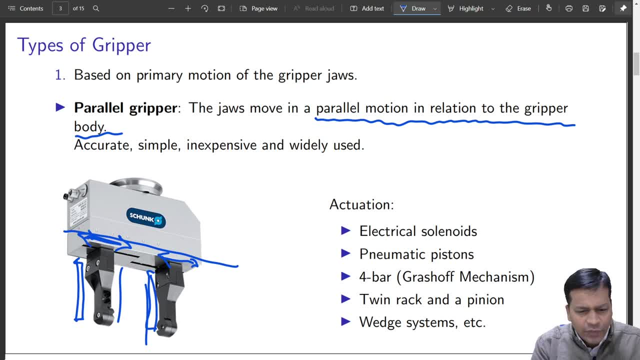 any manipulation that it is doing. They are very, very accurate because you are not giving, you are not changing the angle, you are not changing anything The way it is structured. it is just moved along the direction of internal actuators which are there. 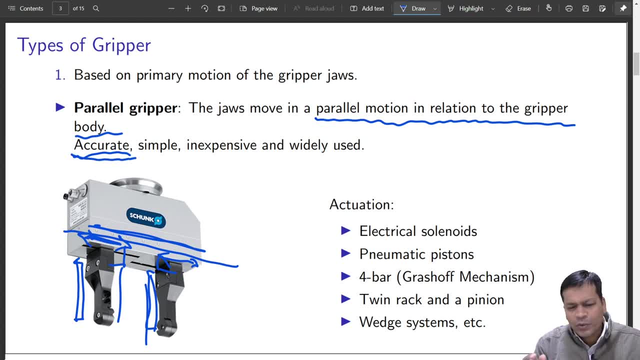 So that is why there is no question of any inaccuracy in this type of thing. So what sort of inaccuracy that can happen in any gripper, Any idea? Yes, backlash. yes, While closing and opening there is a backlash. 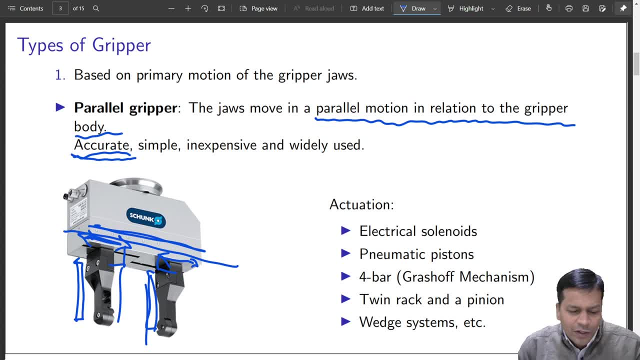 Yes, that is always there. So that can be taken care of easily by having a spring ended gripper while moving at least. for opening it uses spring, For closing it uses some sort of actuator, but for opening it uses spring because you know while opening you are not going to hold anything most of the time. 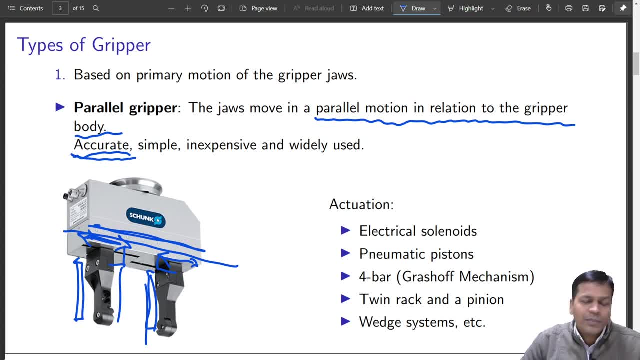 So, yes, you can afford to have that, So that backlash can be eliminated that way. Ok, Another very prominent type of error, inaccuracy, which is there that is found in this type of gripper is it never comes to same distance every time it closes. 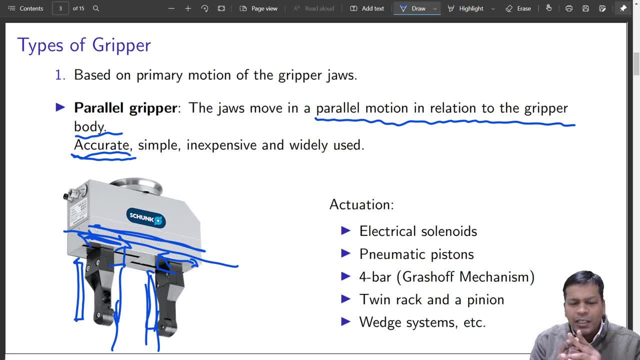 It is not type of backlash. rather it can be inaccuracy in the actuator that drives it, So that can be another one or both. the fingers are not very parallel, Ok, So in that case what will happen? if you hold something, it can fly off. 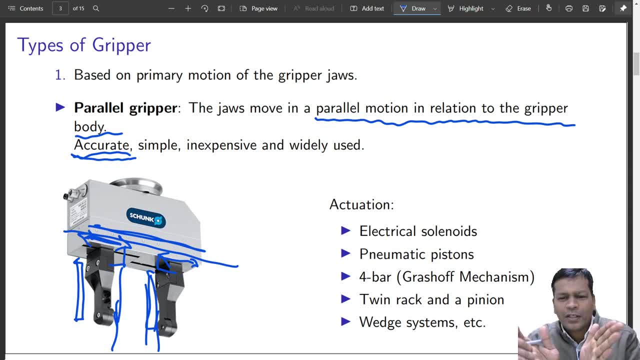 Let us say you are trying to hold a cylinder and your jaws are not like this parallel. rather it is like: opened up, Ok, If it is opened up, what will happen? It will. similarly, if you press it high, it can fly off, Ok. 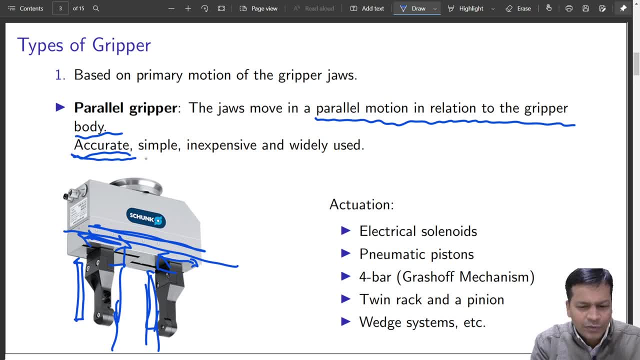 So that should not happen as well. So, more so, these are very, very simple, and because they are simple, directly driven by the actuator, they are inexpensive too, And this is what we are talking about. Ok, This is one of the most widely used type of grippers. 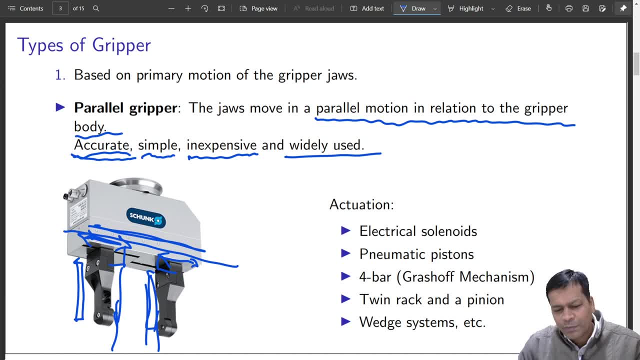 In industry you will find this is the one which is there most of the places, because you can design your end end of this two fingers. design the fingers in such a way so that it can handle multiple objects. So what all ways you can design it may be one of the finger, have a wedge, sort of thing. 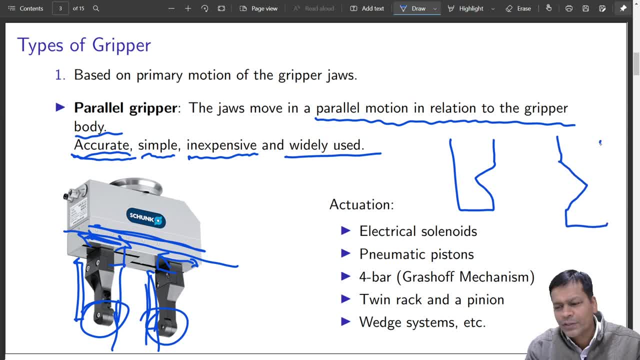 Ok, And another one also has a wedge. so, and both of the finger, both the fingers can move like this. So what will be the advantage of this type of fingers, What you can do with this, Any idea? It can be used in the cylindrical object. 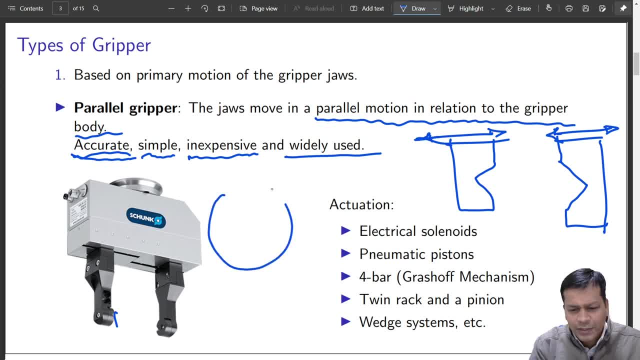 Yes, very good, So you can hold something which is cylindrical using two wedges. Ok, So, yes, Yes, But what happens? No, Most of the time, what you prefer, you would prefer this. a particular size of cylinder will be best fit in this, because that is almost, if you draw a tangent: this finger, this wedge. 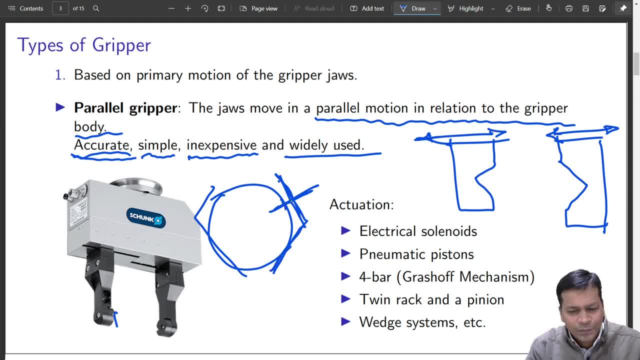 shape is exactly a tangent on this cylinder. Ok, So that would be the best fit. Ok, And if you draw a radial outward, it directly is perpendicular to the wedge. Ok, It is perpendicular to the wedge shape, So that would be the nicest one to have it. 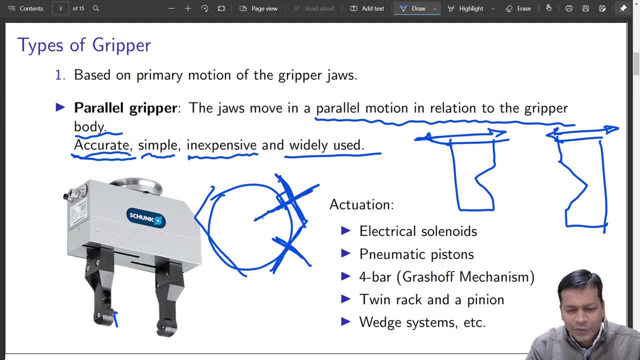 Ok, Best one to have it So it can hold it properly. Ok, So this is something that you can definitely would like to have, But if at all there is change in diameter of this is happening, then same finger will not be suitable. 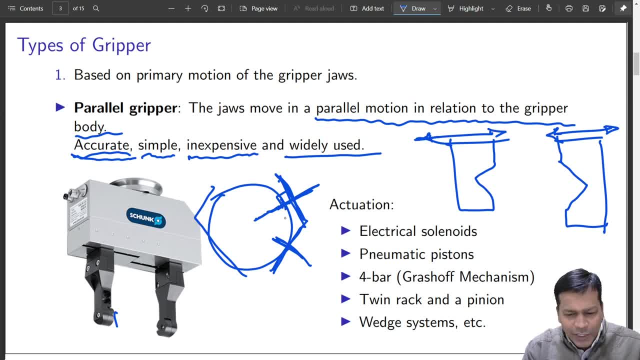 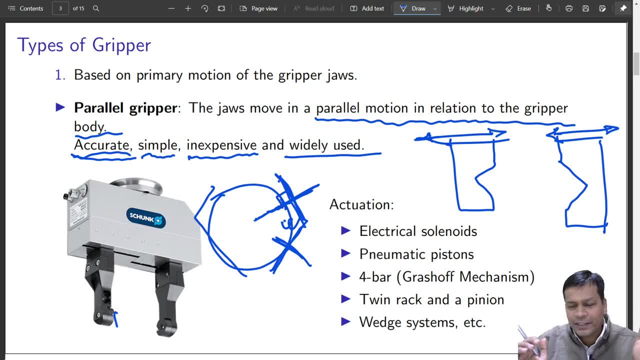 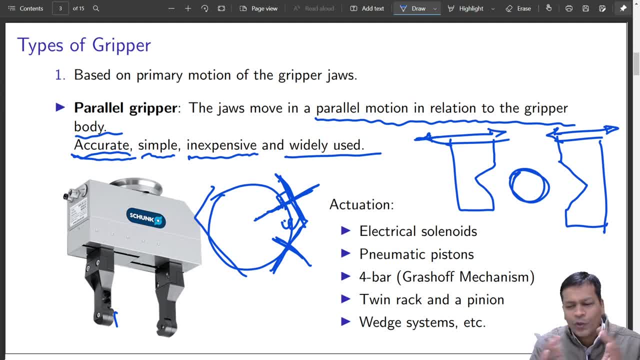 But yes, when ever it will hold, it will hold center aligned, It will. final position of the cylinder will not change What I mean. let us say both the fingers are travelling by simply one. what i mean. what I mean, Ok. 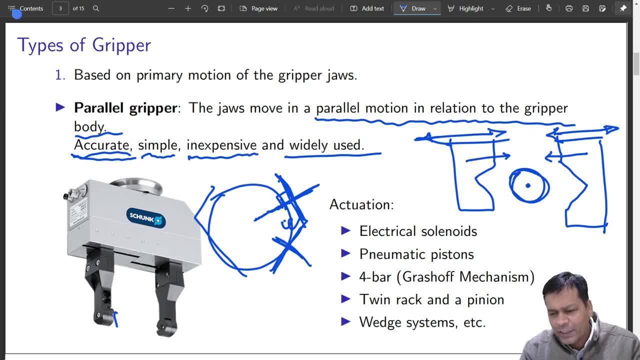 similar distance. finally, wherever they merge together, irrespective of the size of this object, what will happen Every time? the centre will be at the same location, Is it not? Do you agree with me, Yes or no? Take a pause and just try to figure out. You have a wedge. 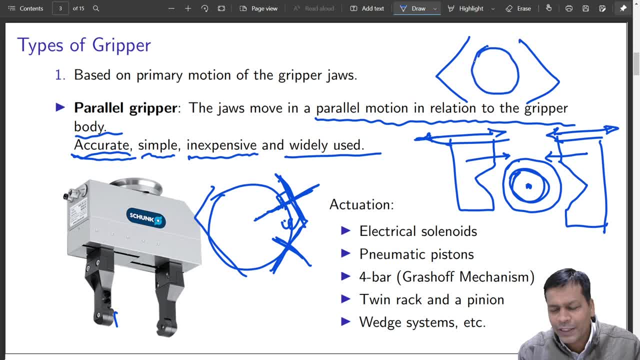 you have another wedge, you want to hold the cylinder, so it will lie here. When it arrived, perfectly in contact with this, it went on like this: Finally, it became like this: So centre. it didn't shift. Wherever it was there, it was here, Even if I change the size of 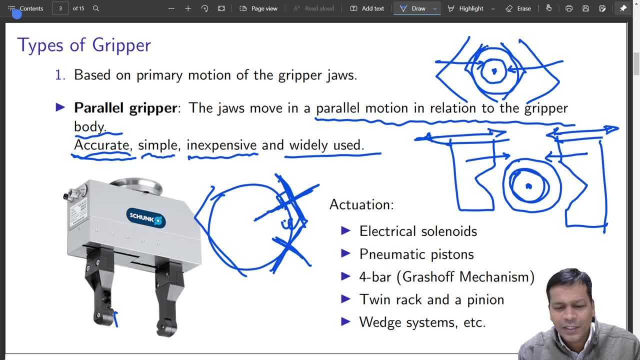 this cylinder. it is not going to change. That means a calibrated position. a calibrated position once it is folded. you know where is the axis of that cylinder, is it not? So axis of cylinder is not going to change. That means you can do a planned movement of this. 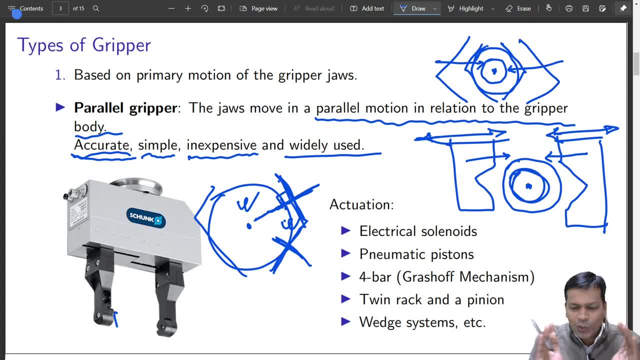 particular cylinder which it holds. It will not just hold it, it can do a. you can precisely manipulate it. That means if you, if at all you, want this cylinder to be inserted to a hole, you can easily do it. If you know the hole location precisely, you can just align. 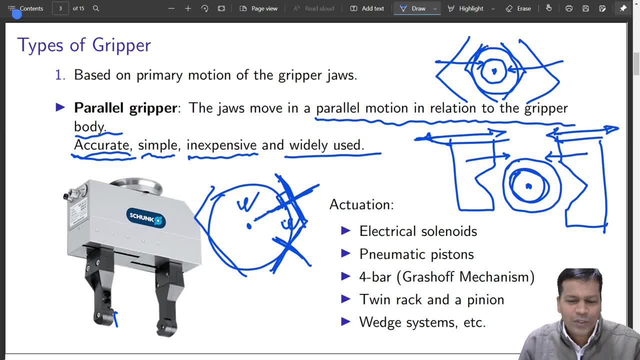 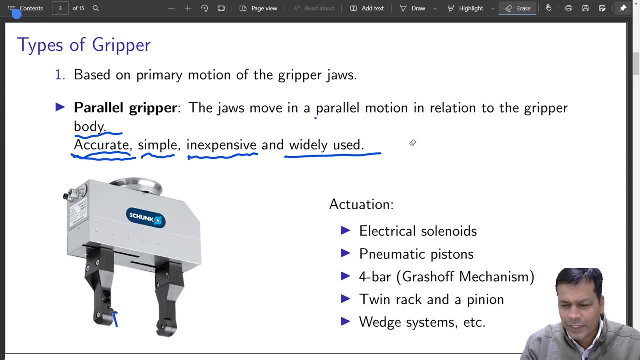 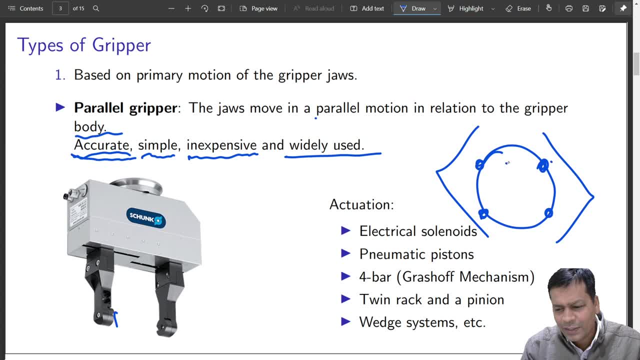 Even the slightest of imperfection in the circular shape of this or in angle of this will cause just three point contact: How many points are required to define a circle? A circle is defined by how many number of points, Minimum 3 points. So 3 are there, If at all. 4th is there that? 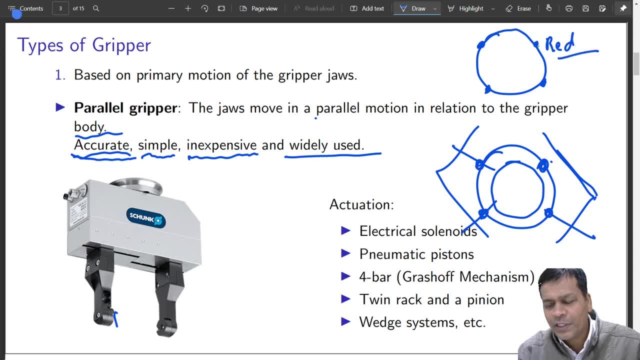 is a redundant one. Even a slight deviation in its position or shape of this will cause losing of contact in one of them, Is it not So? that will be the weakest point: where your object can slip. where your object can slip, Is it not So? 4-point contact is not very. 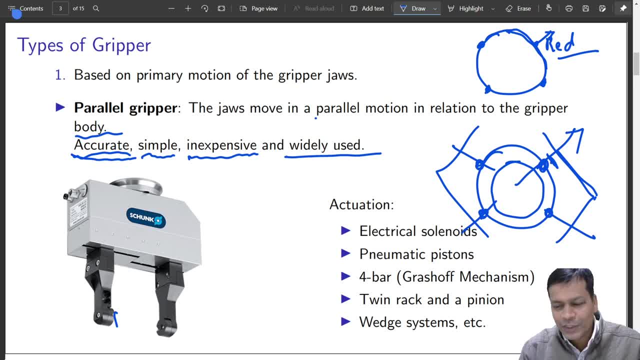 good to hold a cylinder, Although it has a beauty that holding with 4 points all from equal distance from these. finally, it will not change the location of this cylinder. that is fine, But 4-point contact has a probability that one of the contact is not getting established. 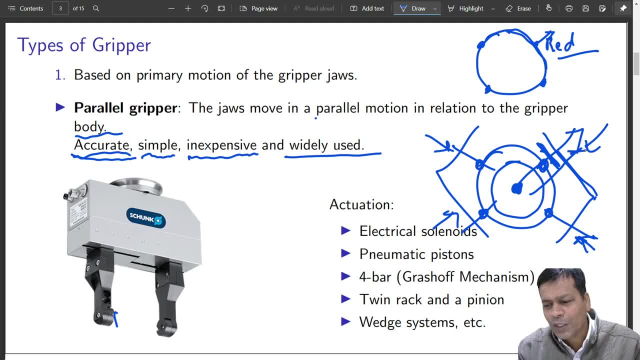 properly and it will not be able to hold a cylinder. It remains loose. So, in order to tackle that, you have a type of gripper when you have one of the fingers as the wedge, other one is just the flat one and both moves. and finally, 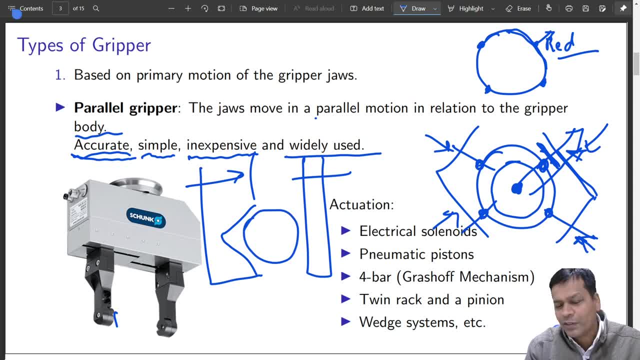 holds a cylindrical object. In this case, how many contacts will be there? How many contacts will be there? 3. Yes, one is here, another one here, another one here, and you can precisely define the contact. So, in this case, how many contacts will be there? 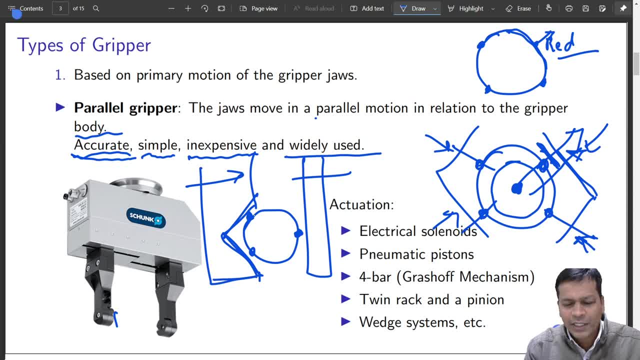 You can precisely define your finger wedge shape so as to make a proper contacts, so that it does not fly out. Problem with this is center will shift when you hold this object. Different size of cylinder will have center located at a different location, Is it not? 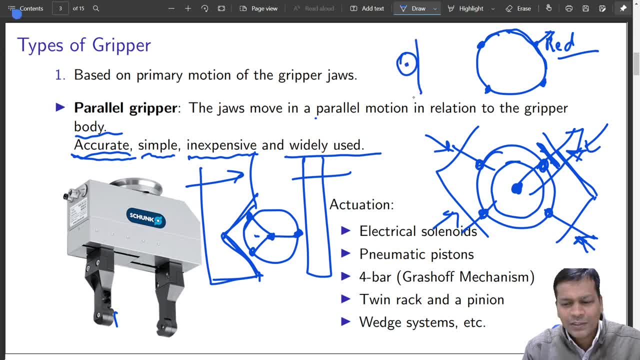 So different circular shape. this will be the radius distance. this will come like this, so this distance will vary. the center line of the cylinder will vary by amount, which is equal to radius from the flat finger, Is it not? So that is why this changes. okay. 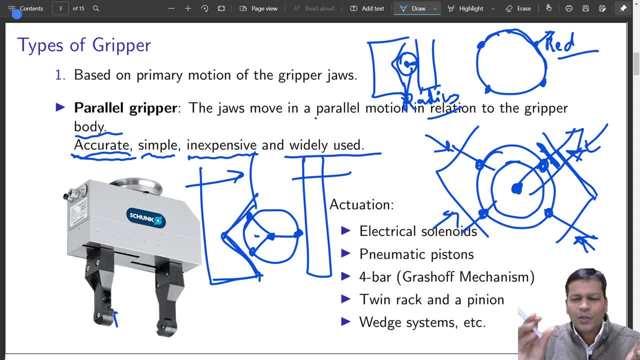 So every time you hold a different cylinder it is holded at a different location, So it becomes very difficult to precisely insert this. if at all it has to be inserted to a hole. You don't know the axis because radii are changing. okay, 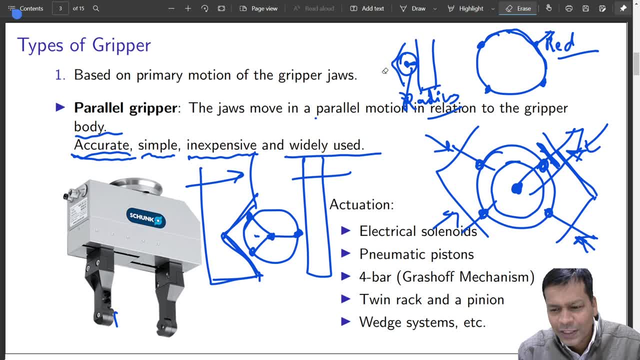 So that is the reason three finger has its own advantage: wedge on one side and flat on the other one. yes, it can hold it firmly because it is circular. if at all you target to hold a circular object, This is the best one because it is making a three point contact. but if it is to be moved, 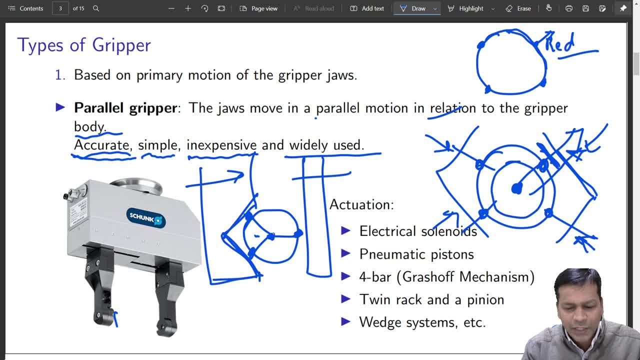 precisely to some other location. yes, it can cause some error because diameters- this radius- can change and axis can also change, So there are different pros and cons. So you now got the idea. so parallel finger can be used to grasp multiple diameter objects. 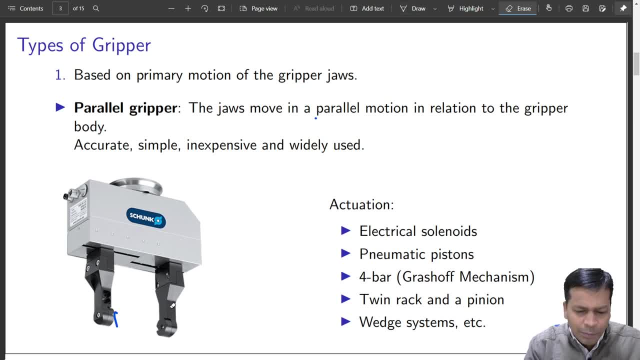 not just diameter objects. you can have rubber padded. these places can be rubber padded so that you can grasp multiple sized objects, and it should not. it won't slip also okay. So there is there is some inherent advantage of this. it is widely applied parallel fingers. 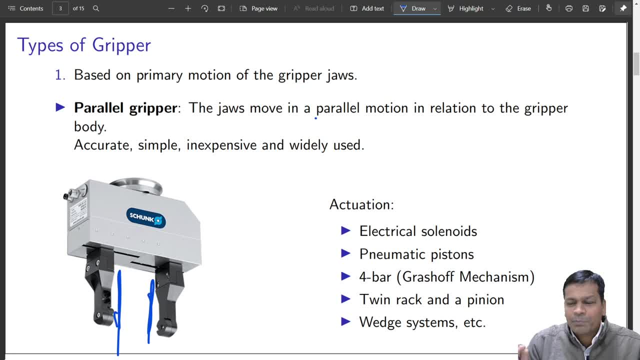 are widely applied. okay, and you can hold multiple things. So you now got one more idea. one more idea that it can. it can hold multiple objects, first of all, And yes, please do not make noise go off, actually, So anyway. so, yes, you can at least fit a pad. you can at least fit a pad here, hold multiple. 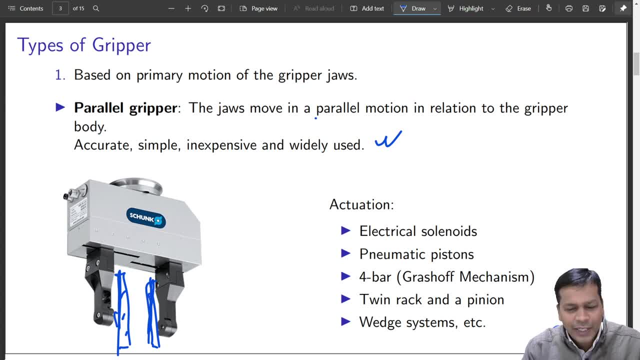 sized object. okay, it does not slip off and it is very easy to work off with, okay. So these, these are some of the advantages. So, actuation wise, yes, it has. it can run on electrical solenoids or pneumatic solenoids. 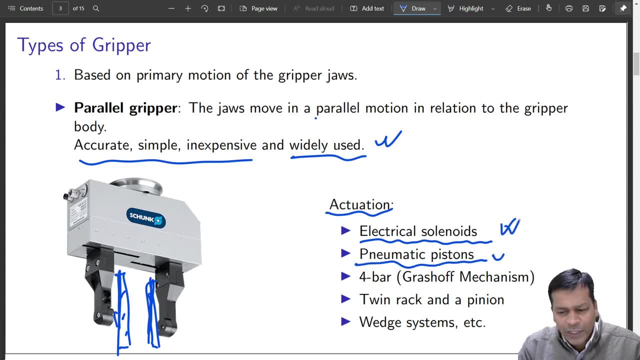 You have seen both of them by now, because you have already seen multiple types of actuators, So you can have electrical solenoids that move these two fingers. okay, In both the cases, you can have natural compliance. What is natural compliance? 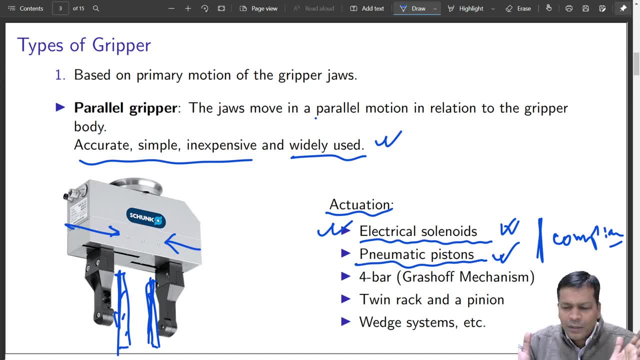 If it is a pneumatic one, you know, after you hold something you cannot elevate the pressure. okay, If you have a pressure which is fixed in that line, you cannot cannot apply force more than something, right? So if you can control the force of gripping force by controlling the pressure of the pneumatic, 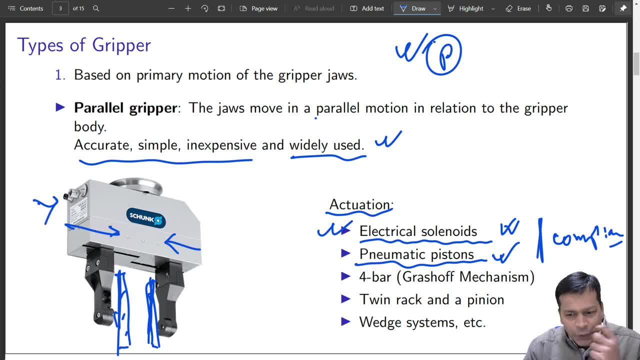 line that goes to this: okay, So they are. they are compliant. they are naturally cushion type. it won't crush something. okay. Four bar mechanism. Grashof's mechanism: I will show you in the next slide. twin rack. 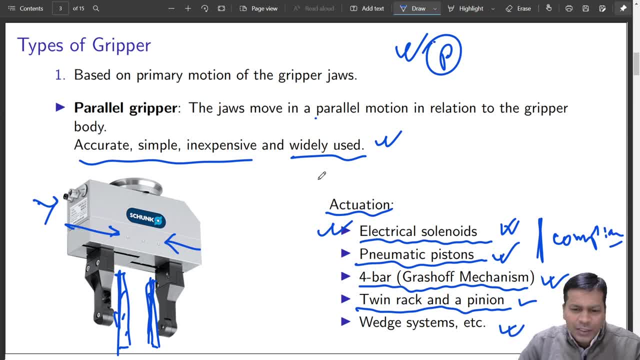 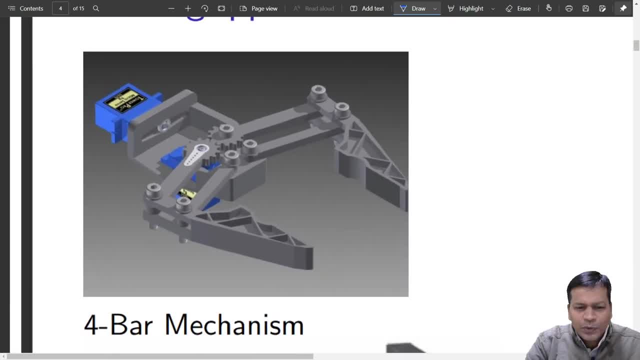 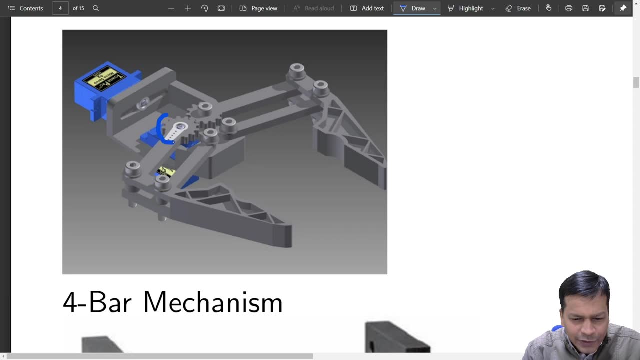 and a piston mechanism. Okay, These are some of the types of this type of gripper. okay, So here it goes. So it is a four bar mechanism. hope you can understand how it will work, right? So this is one of the gear that rotates. 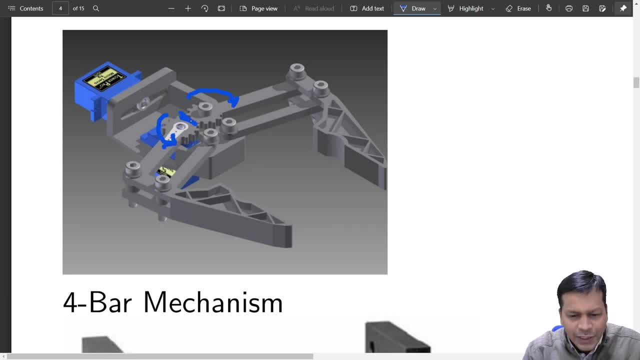 If this rotates, that will also rotate, because there is a gear meshing which is here, And both of them- this is a four bar mechanism, right? If one of the arm? So it is a four bar mechanism. If one of the arm rotates, this also will rotate. this will move like this, is it not? 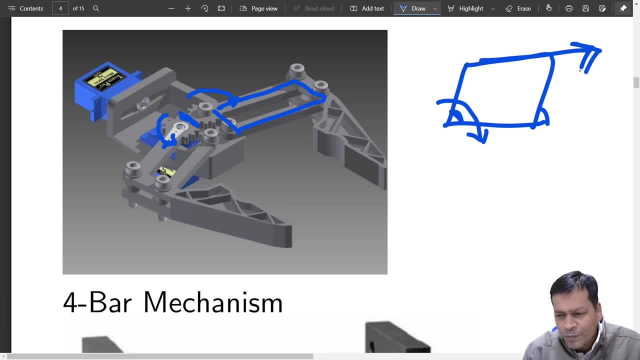 So that makes it move like this, as well as because this height will go closer after this, this distance will, as you move this actuator, it not just goes this direction, it also comes closer. So that is making these two fingers come closer. 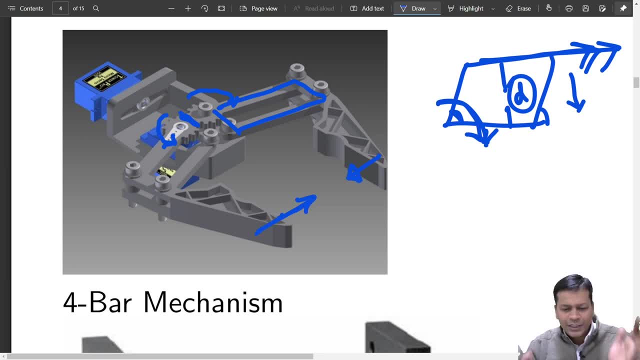 Okay, So it will move. It will move like this. So, yes, this type of arm is very, very simple. It can apply quite good amount of gripping force. Only problem that I see here is, yes, you have a circular surface at both the ends. 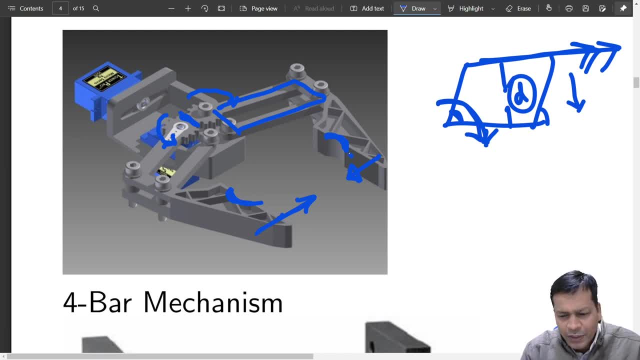 so that it can grasp something which is cylindrical. If not, then it is rubber padded also. you can hold any diameter object also, it won't slip. But yes, apart from moving the jaws like this, It is also travelling in this direction. 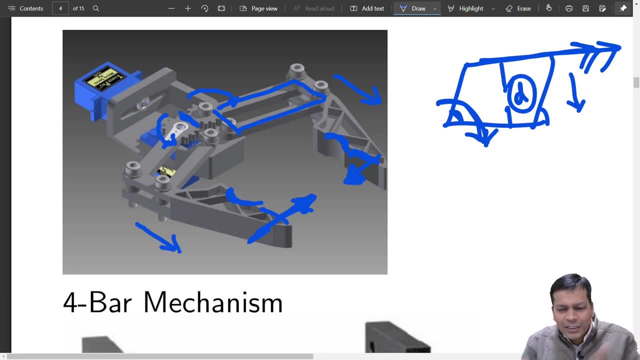 That is not always desired. It is very difficult to estimate where you are going to end up. Okay It is. it has a probability to hit the target right, If at all it is approached from the top. there is a frame which is here on which there is: 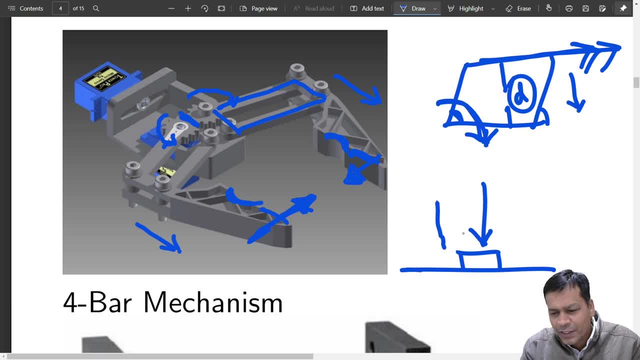 an object you want to hold and your fingers are not just moving like this, rather it is also moving towards the object while closing. So you can help it, Okay, Okay. So you can hit this object very easily. So that is the problem with this type of things. or you can even hit the table on which it. 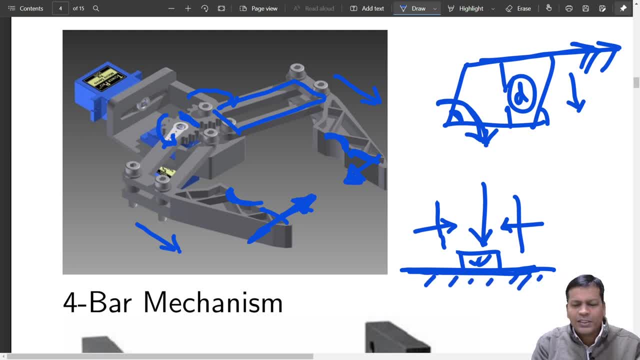 is kept. So this is the problem with this. but yes, sideways it can move very easily. Okay, And very, very simple: just one actuator that drives it and both the fingers they travel with same amount of distance, Okay. 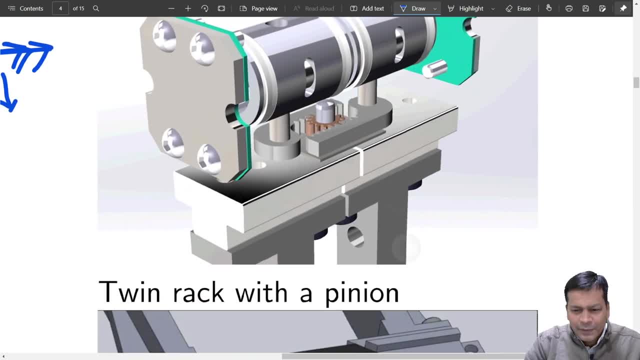 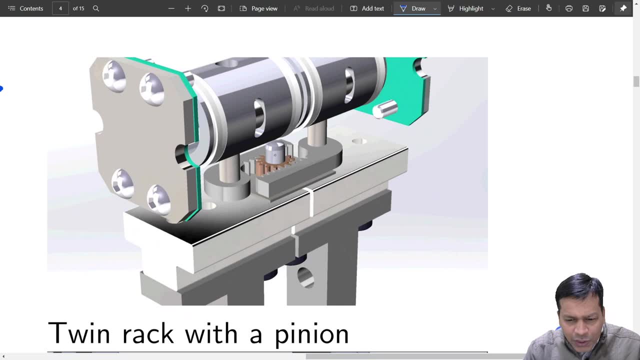 So this is one of them. Another one is a similar one. When you have Okay, I will zoom it further. Yes, Hope you can see it. So this is a gear which is here. Okay, If this shaft rotates, one of them will move like this, another one will move like this: 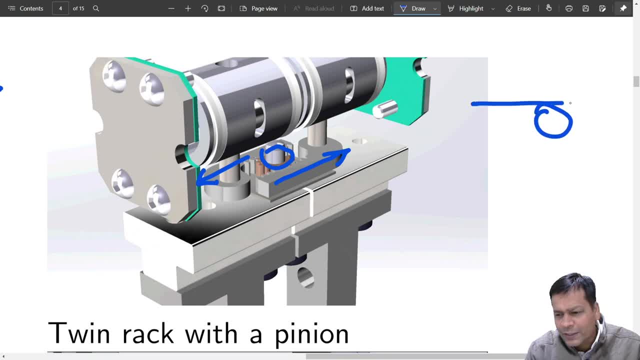 If it rotates in counter. so actually it is something like this: You have a rack, you have a rack like this, Okay, And fingers are attached to both of them, Okay. So if you, if this shaft, rotates like this, what will happen? 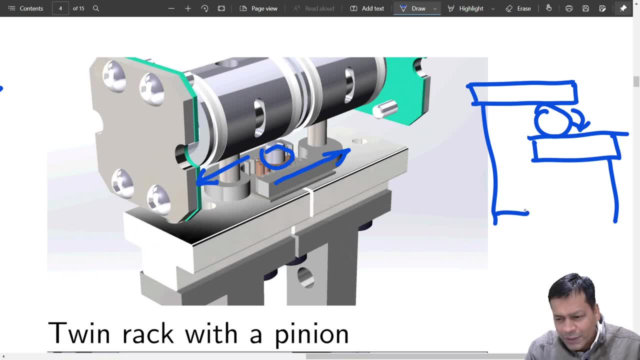 Both the fingers will come Closer, Is it not? Both will come closer. If it rotates in counter clockwise direction, what will happen? It will go further apart. So that is opening. So this is twin rack and a pinion based arrangement. 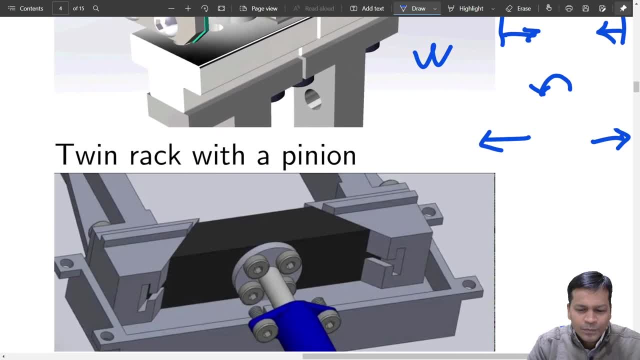 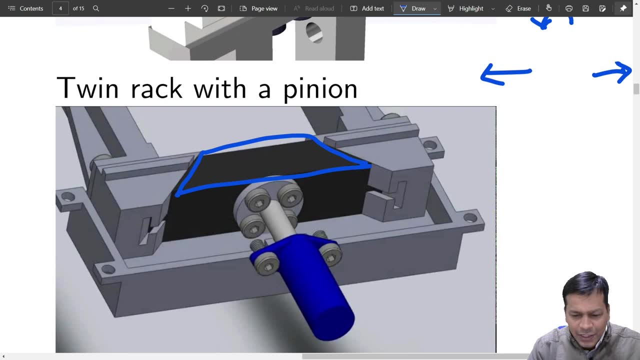 This is also quite common. This is also a parallel finger gripper. Okay, What is this? This is a wedge. This is a wedge. Right, You can see this. This is a pneumatic cylinder which can push and pull this particular element. 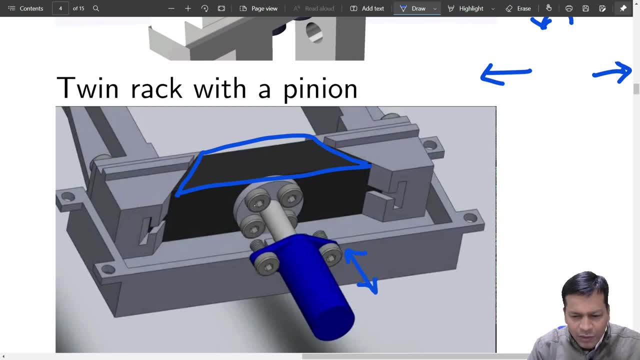 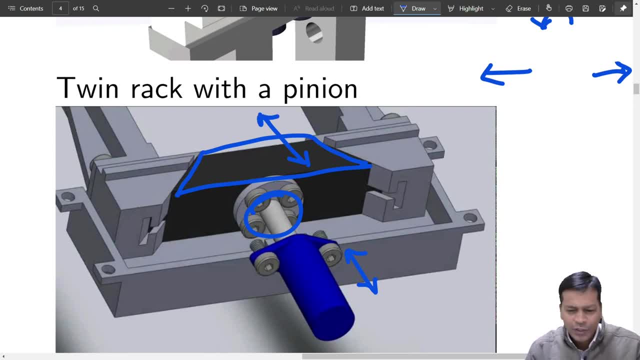 Okay, It can either go in or it can go out, Right? So just one actuator and you have two sliding wedges. So once it gets inserted, these two will go apart, Is it not? So if you pull it out, what will happen? 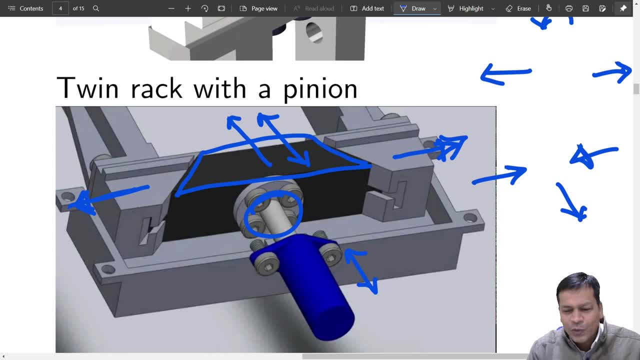 They will come closer. Okay, So you can do opening and closing. So it is run by a spring ring that brings it closer when this wedge is taken out. so it is a spring driven from here. So this is another mechanism also which can do a similar parallel fingered operation and 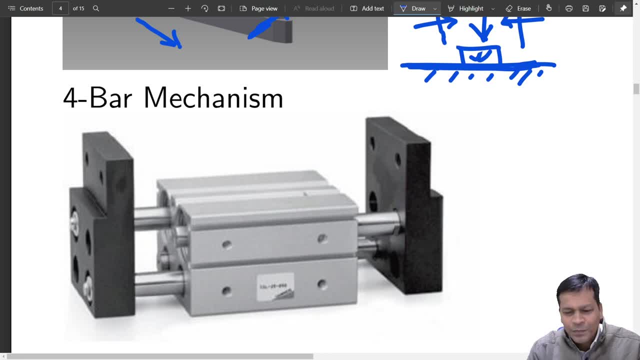 then there are twin cylinder thing, so you have a pneumatic cylinder which makes this actuator out, in and out, and there is another one, also two cylinders, doing this job. But yes, both the travels may be little different travel. you cannot guarantee that both of them. 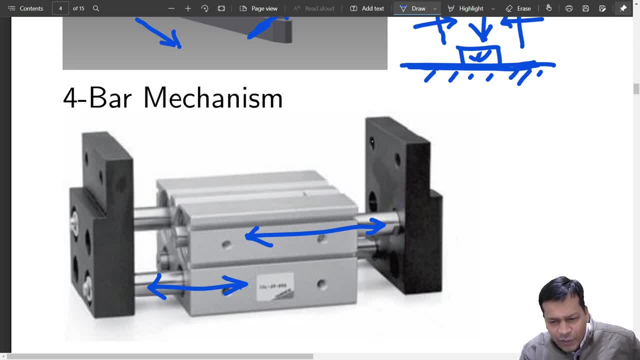 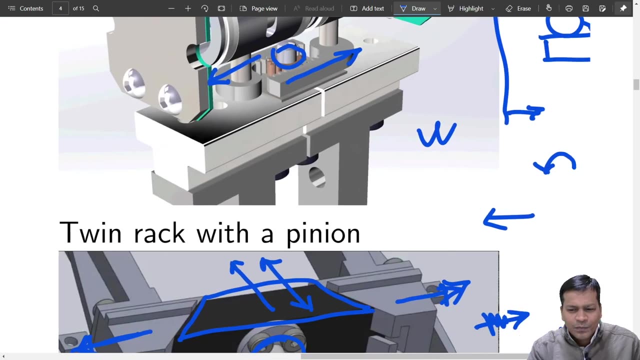 will travel by same amount of distance. if this will face more resistance, definitely this will travel less. if this faces more resistance, this will travel less. so travel is independent because both the cylinders are different, but in this case, this case, or this case, travel is guaranteed that they are going to be same. 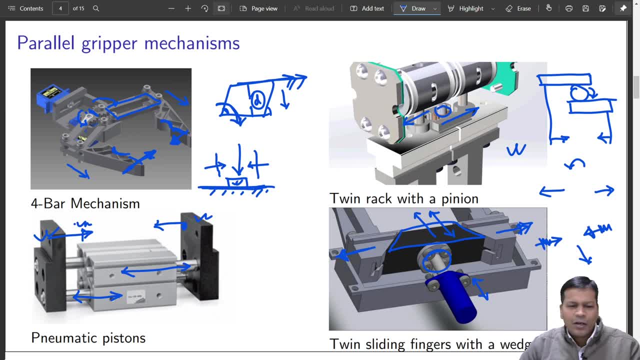 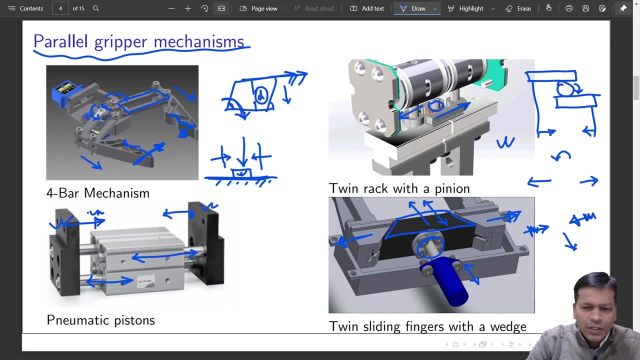 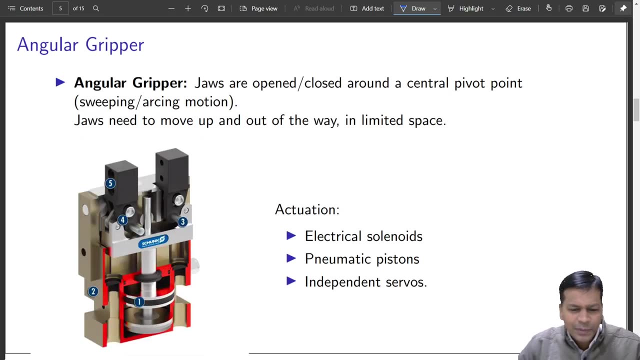 So these are the two mechanisms. So these are four major types of operations of parallel fingered mechanism. that is a gripper. So next one is angular gripper. What is an angular gripper In this case? what you see, jaws are opened or closed around a central pivot, around a 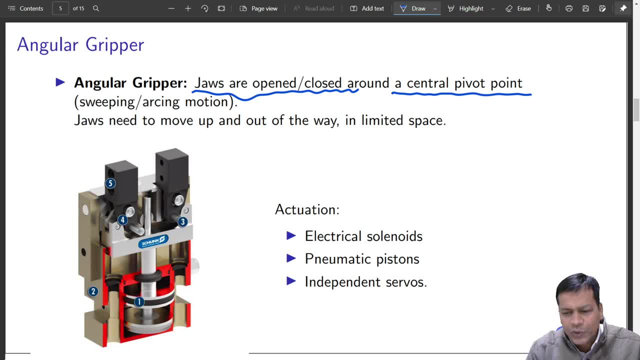 central pivot, sweeping or in arcing motion. That means initially the finger. That means initially the finger. The fingers were like this: in a closed position. If at all it opens up, it will open up like in the same point. it will turn up like this: 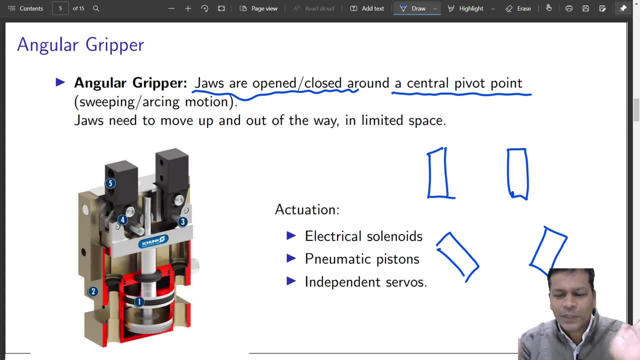 That is opening, So closing and opening, closing and opening so you can hold something like this: So, while closing, if it sees a bigger size cylinder, it can make this fly off, is it not? So in order to handle that, 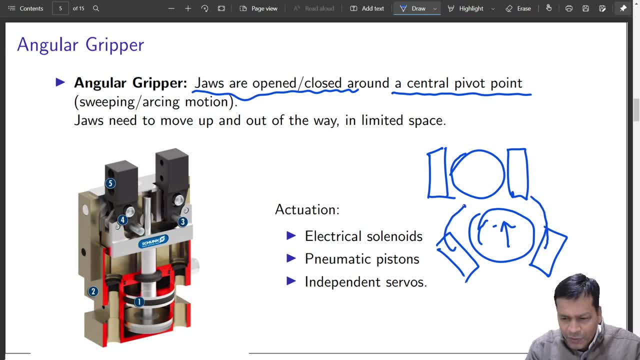 You have something which is known as Enveloping attachment. You have an attachment which is acting like an enveloping grasp, So your fingers are moving in an angular fashion, But now you have it is not just two fingers which are going to move. 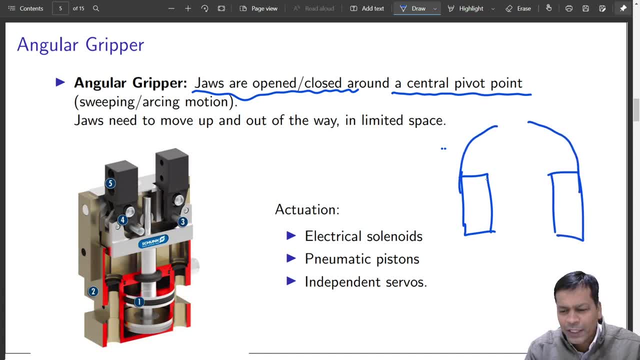 You also have attachment, which is something like this: So finally, you have an attachment on top of two moving fingers, So that is what is called an enveloping grasp. Okay, If you hold something which is cylindrical, or even a square one, it should not slip out. 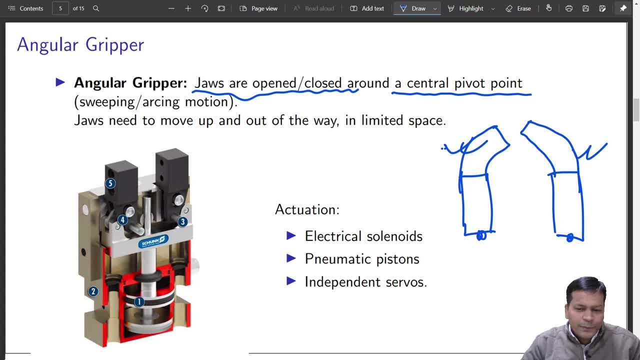 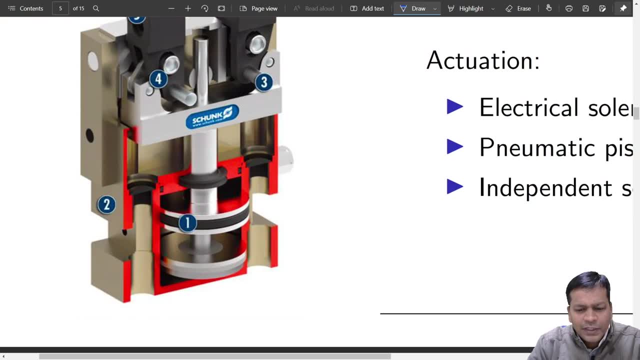 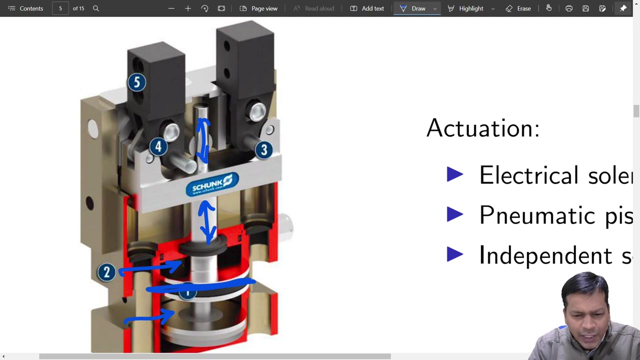 while you were closing. So jaws need to so effectively what you see, you have a, you have a cylinder, you have a pneumatic cylinder. you can pump in air from here. you can pump in air here so that this can travel in and out and effectively, that is the one which is moving this and I 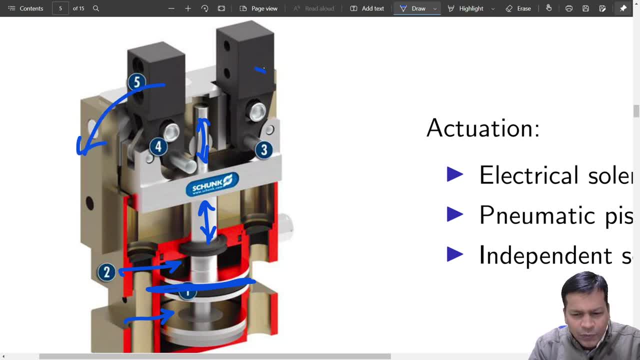 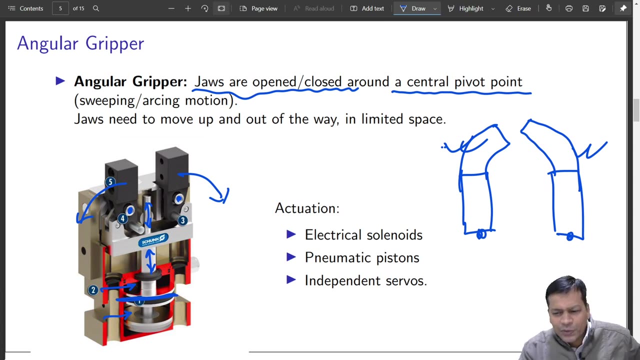 can. ultimately, you can move this out or in, so this is your pivot. this is your pivot, So this is how it operates. So, yes, this is very, very popular and widely used. again, both the fingers will travel similarly, but you need an arrangement like this which makes it quite safe also. yes, so because 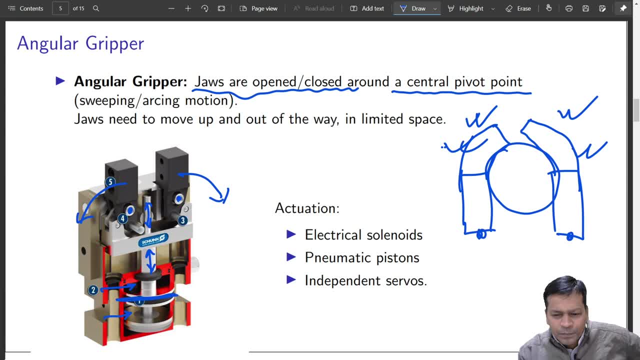 it can envelope, which is grasped. Even in case of parallel finger, you can have this type of arrangement, okay. So there are various ways this can operate, but this is very, very quick because it is not linear motion when this is moved in a straight line, in a linear fashion. the closing. 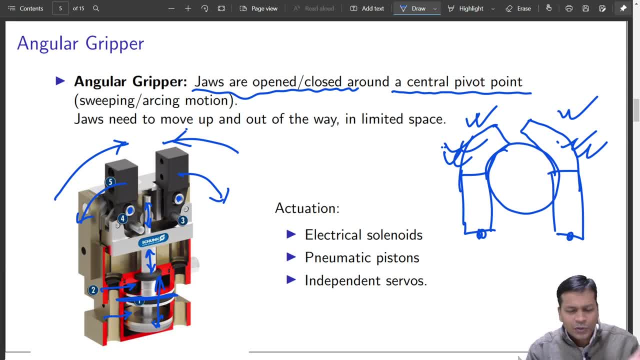 is not linear. linear means it is not proportional, so as it goes closer, it becomes faster, okay. So this, this is very, very faster in operation. Actuation wise, This also can be electrical, solenoid, pneumatic pistons or independent servos. 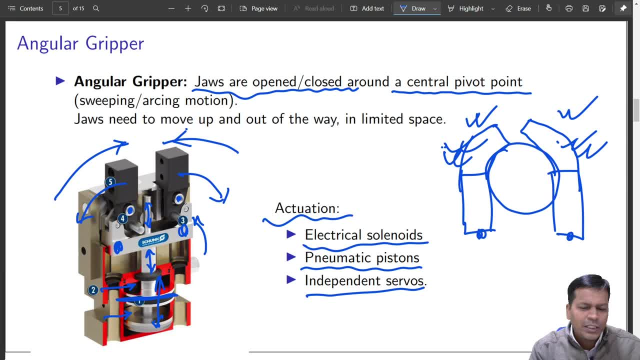 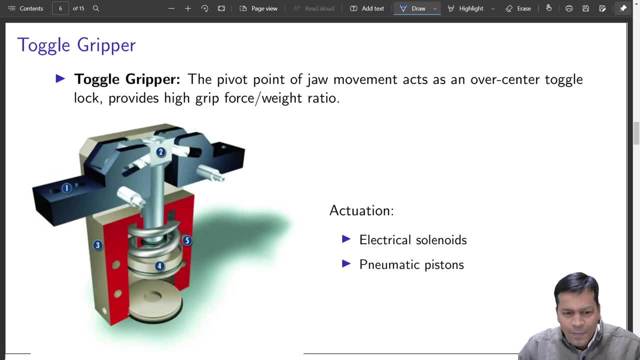 You can have a servo here. you can have a servo here which independently closes both the fingers right. So that is an angular gripper. and then you have a toggle gripper. this is a unique type of angular gripper which is toggle position. that means, once it is closed, it cannot be. 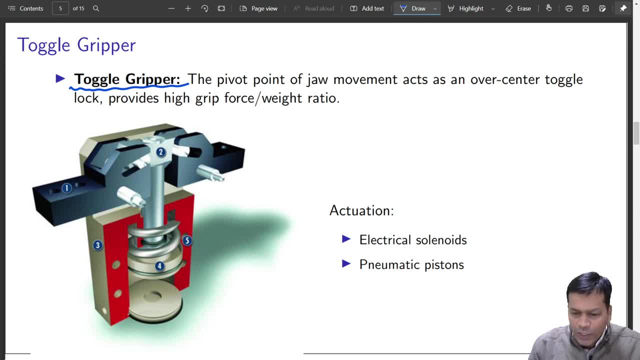 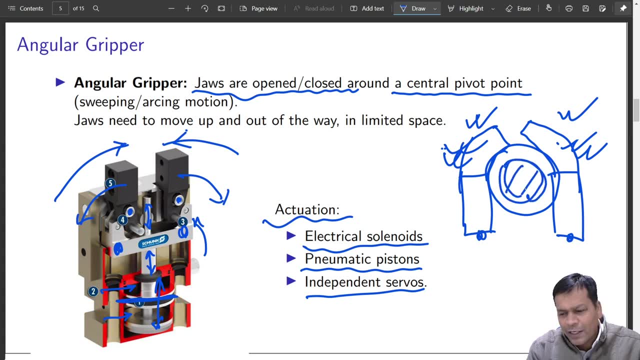 opened up Until and unless you. so what was wrong in this? if this object, this object, applies a force in opposite direction, what will happen? these fingers will open up because there is no locking mechanism. okay, Once it is, it can be opened. that means it is back drivable. 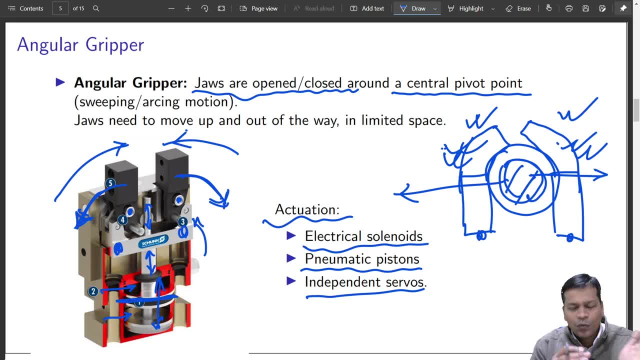 Fingers are back drivable. So what happens? So, while you are in motion, You can have inertial forces arising out of motion. if this object that it is holding is very, very heavy, that can apply inertial loads on these fingers and your finger can. 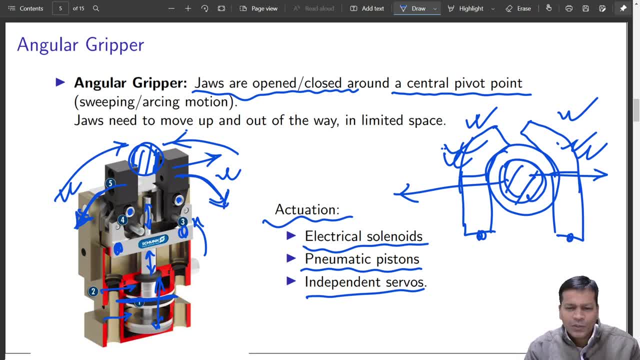 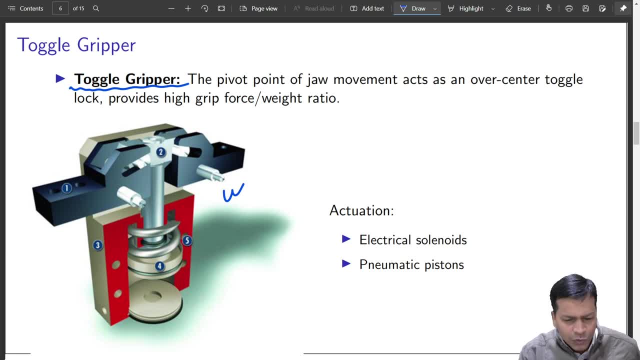 be little slackened if not open. okay, So that was the problem with this. So this is not the problem with this type of gripper. that is a toggle gripper, So in whatever position it is, this also opens and closes in an angular way. 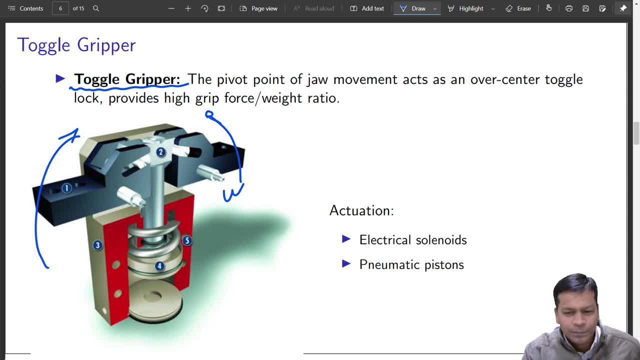 But wherever it is okay. it locks. in its position, The pivot point of joy movement acts like a over-centred toggle toggle lock. over-centred toggle lock. You can imagine if you pull it out this will further get into these slots okay. 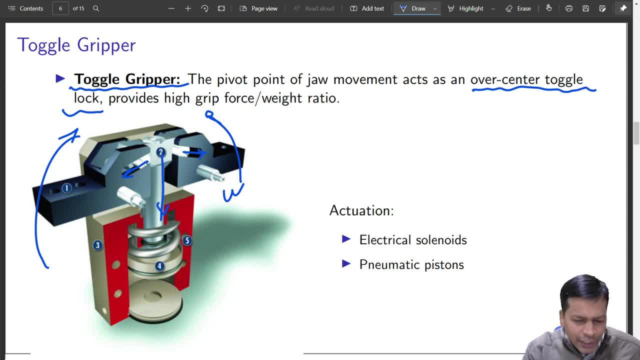 That provides it in a locking way. So until and unless you provide force from this actuator. actuator is like you have a spring to return Air to open it up. You apply air pressure, it will open. These will go wider open, okay. 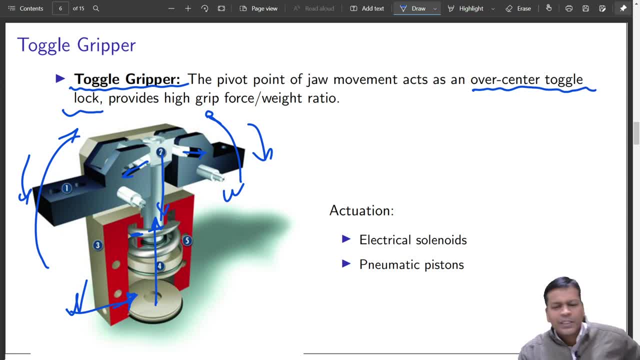 If you just release this air, it will automatically close and it will be in a locked state. It can be electrical, it can be pneumatic. It is not independently servoed by okay. It provides a high gripping force, So force by weight ratio. 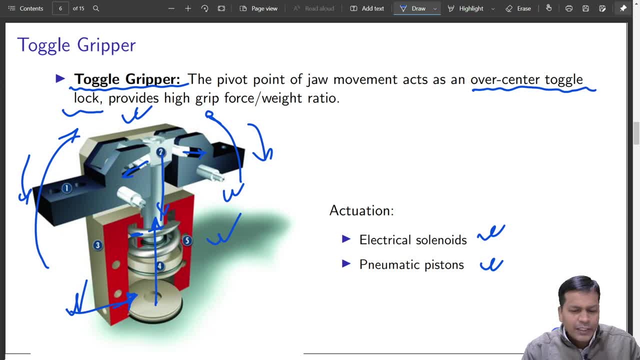 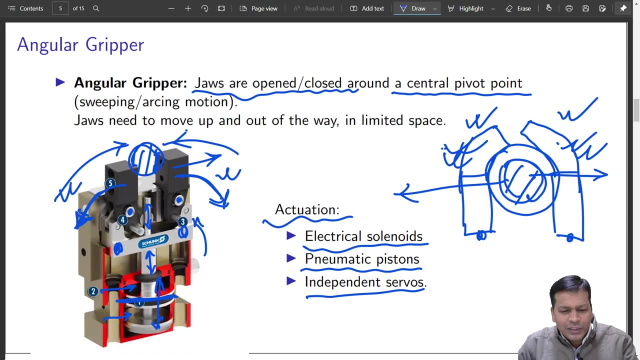 Of this type of gripper is very, very high, widely used again. So why not use the best one? Why should we switch from this to this? So what is the problem with this? Why should we go for this one? What is the problem with this? so that we can switch for this one also. 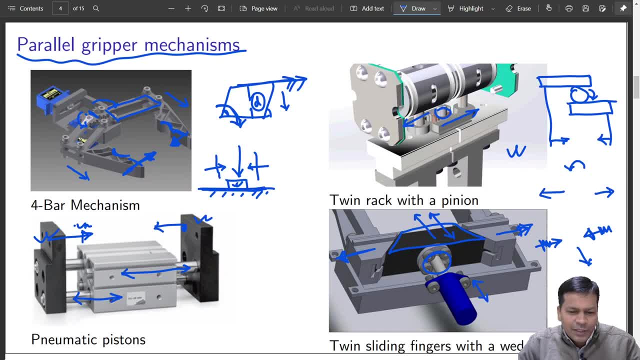 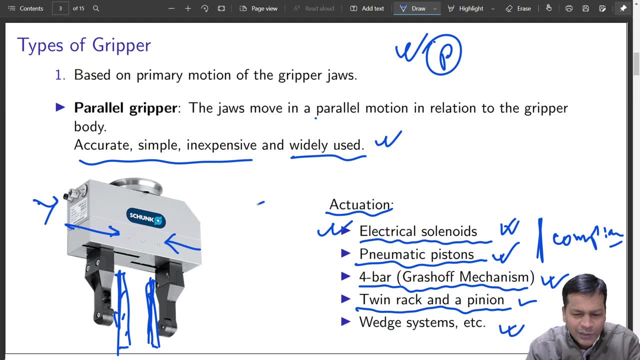 Okay, So there are different pros and cons in each of them. As I have said, in case of parallel mechanism, there are various approaches. you can do. This is the best one. You can have a V or a plat. You can have V and a V. You can have semicircular and a semicircular of different sizes. 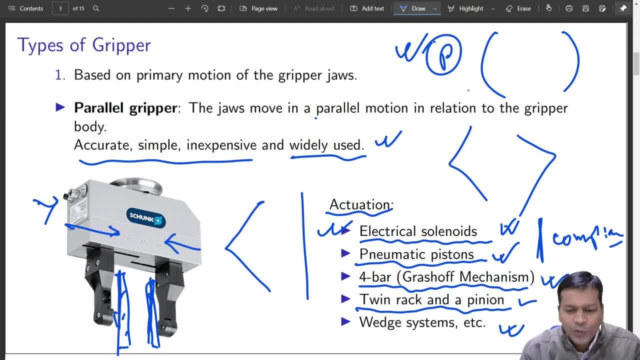 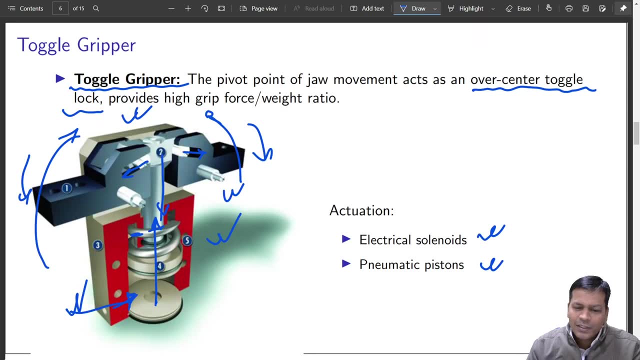 So different object, different, different object can be holded. You now know a philosophy of a gripper. Every gripper is unique by its application, by its application, okay. So that is the reason: Application demands a particular type of gripper. 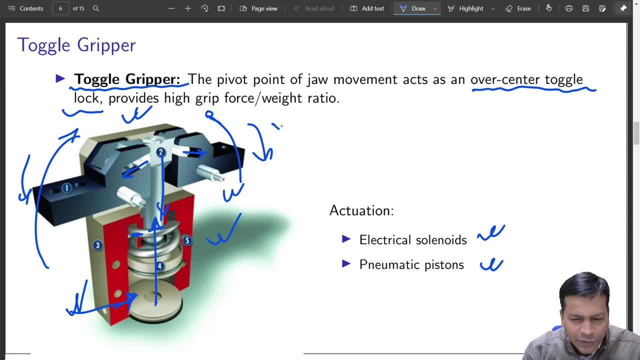 If at all. you do not need a locked gripper. You can have V or a plat, You can have V and a V, You can have semicircular and a semicircular of different sizes. So there is a problem. If you are using a locking thing, why should you lock it first of all? 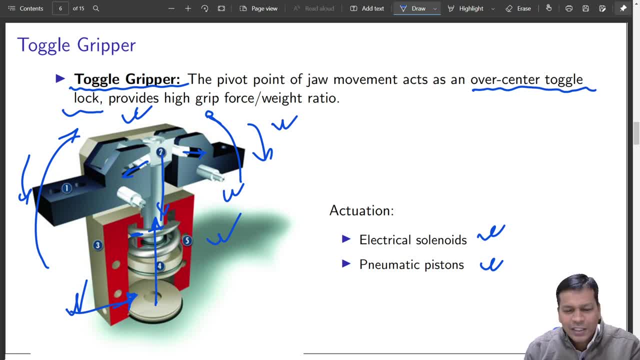 What is wrong in locking something, even if it does not demand locking? So there are pros and cons with this also. Okay. So once it is locked, it is locked. Problem is, it is not compliant. It is not compliant. You are removing the, you are removing the air and it is closing using a spring pressure. 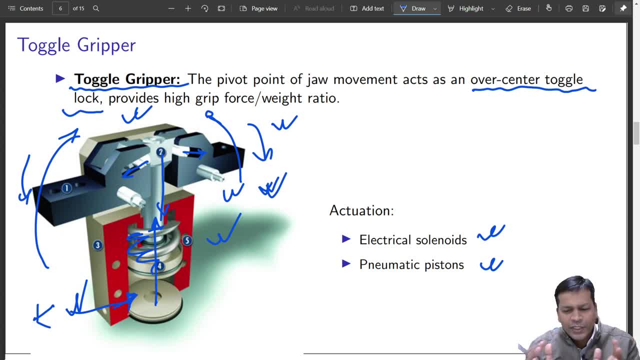 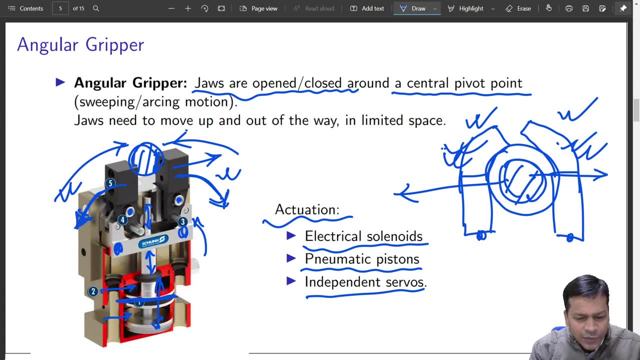 So closing force is always constant, So you have different types of object, So it can be locked, So it cannot handle multiple types of objects, whereas this can. You can adjust the air pressure and you can have multiple forces in order to grip something. 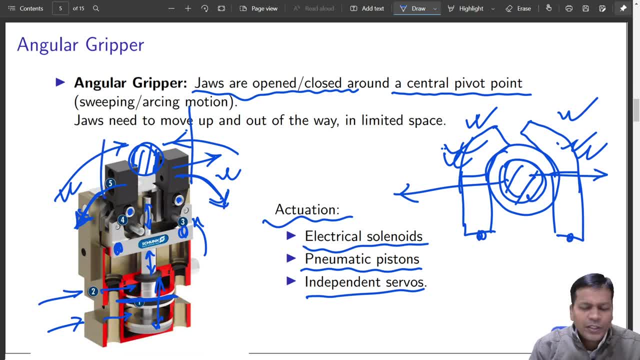 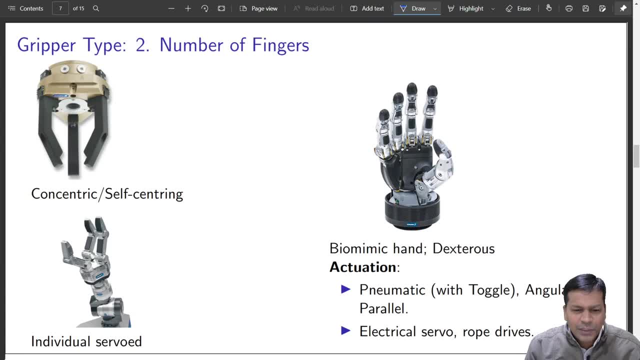 and, moreover, you can attach different types of enclosing in order to envelop something. So those things are missing. yes, based on number of rippers. also based on, this is type number 2, that is based on the gripper type, that is, number of fingers. 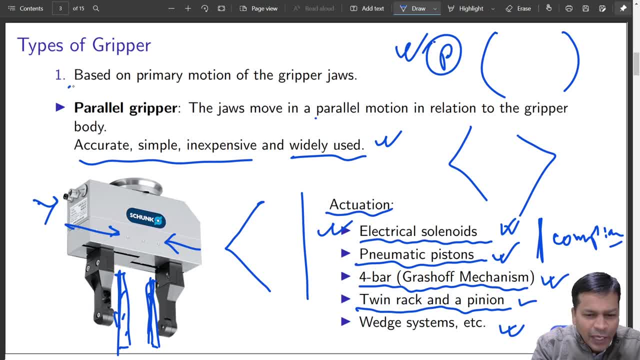 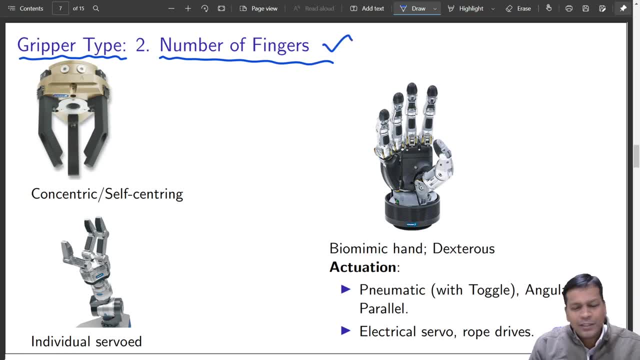 So far, you have seen what, Based on the primary motion of the gripper jaws, this is number of fingers you can also classify. So this is a three fingered one. Each finger can have something like circular shape or it can have a wedge like this. so 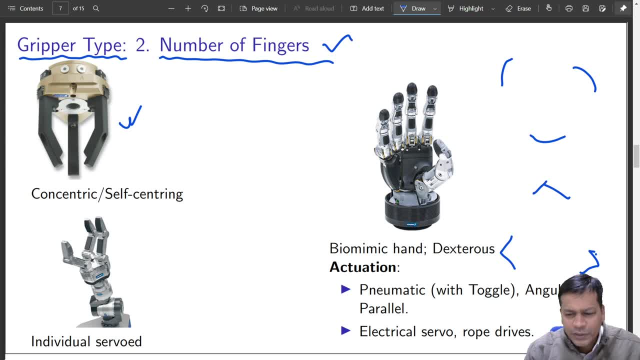 as to hold multiple point contraptions. So this is a three fingered one. it is a self centering also that. what does it mean? Have you seen a chuck of a lathe? So what is the point in using three fingered and a four fingered one? 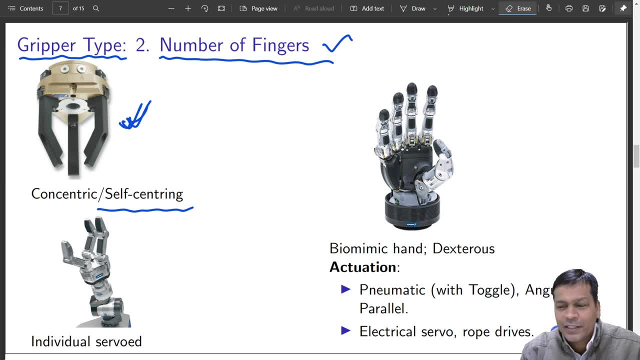 Self centering, because you want it to be self centred, So same is there. Same is the duty of this type of gripper. Every time, all the fingers, they travel with the same distance when it moves and a cylindrical surface of multiple diameter can be folded properly, and every time it holds different. 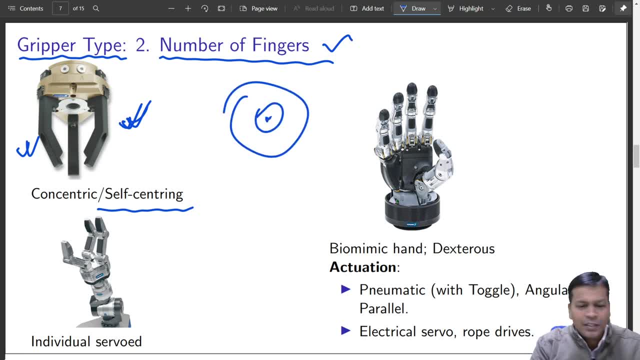 diameter centre will be at the same location, may be at the axis of this gripper, So you can precisely pick from a place and put it in the another place. Same benefit, as we had it in a parallel fingered gripper which was something like this, is it? 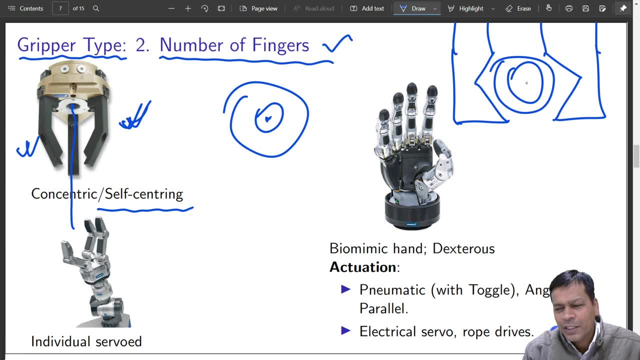 not, So every time it will hold different diameter. centre will remain there. But yes, you saw there is a problem of four point gripping, so this is a three point gripping and self centering also. So, yes, this is, but this is very, very expensive. 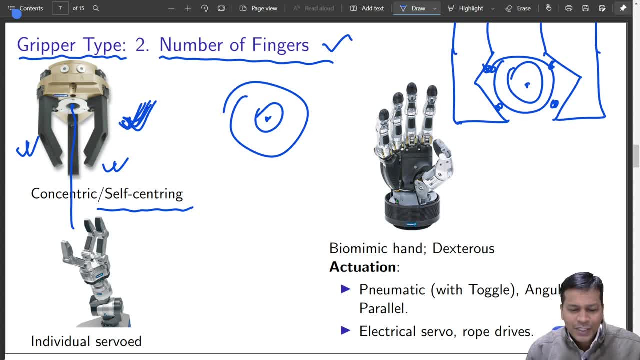 Number of fingers. they counts to your price also. Ok, Ok, That is fine, very good, No, no, no, I do not need it now. I will definitely ask you when required. Ok So, but now I think you have to just keep on following what I am telling. first, 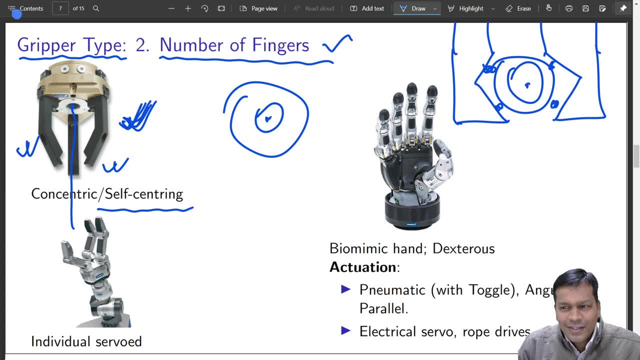 Ok, Definitely, I will ask you. Do not worry, If you have done it, it is very good. Ok, May be in one of the class you demonstrate after this class what you have done. Ok, Ok, Thank you. 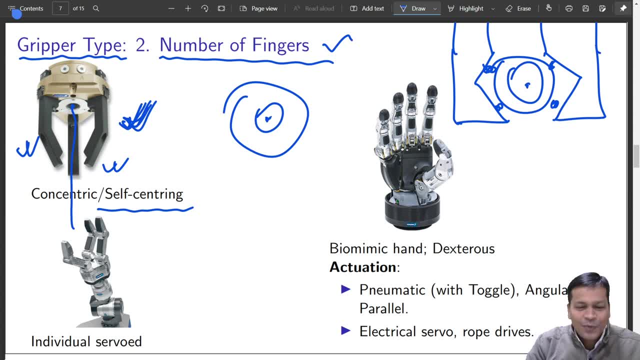 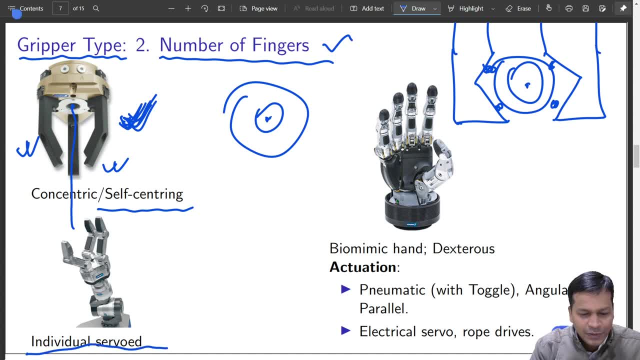 Thank you, Ok, Maybe tomorrow sometime. Ok, so this is an individually servoed one. Individually servoed one means each of the finger, each of the finger is individually servoed. Ok, so you can adjust. it is more dexterous. 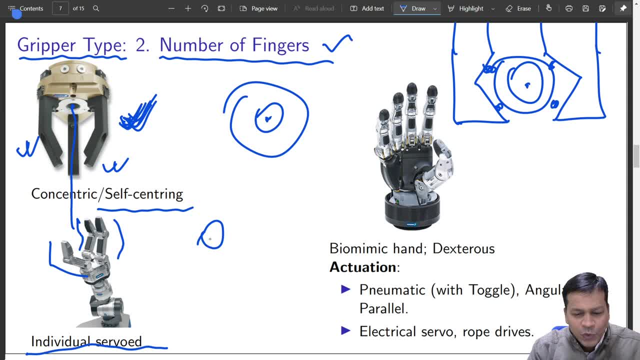 That means for a given object, you can have the object location with respect to this wrist at different place. Ok, You can maneuver precisely the wrist. Ok, your object with respect to the wrist. also, That is not the freedom with this or with a two-fingered gripper or an angular gripper. 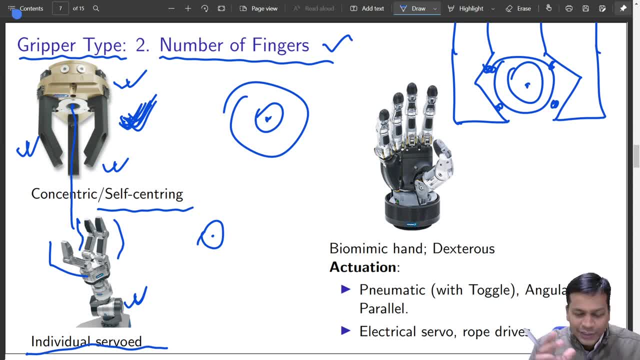 or any other earlier gripper that we have seen. So what this can do: it can orient something if it is holding something, like the way you are holding your pen you normally hold with three fingers, you can precisely move this pen with respect to your wrist so that you can do small manipulations also. 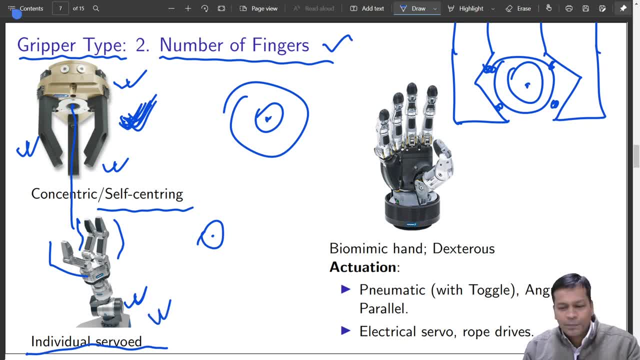 That is what is possible with this type of gripper. So more finger, better it is, But expensive they are. So there is an arm hand which is known as biomimic hand. Why biomimic? It mostly resembles to your own arm, your own palm. 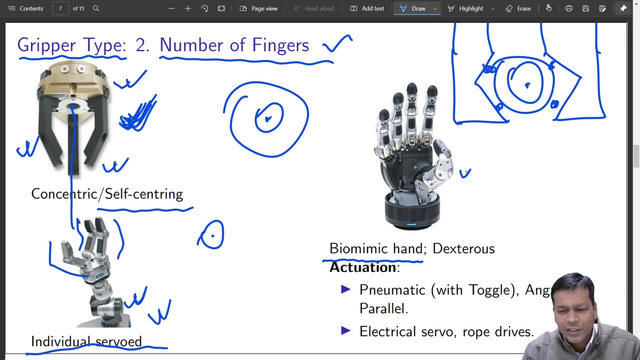 So everything is like this. number of fingers are also this, Degrees of freedom are also matching. At the same time it has tactile sensors over here which can even detect slipping. They are very, very dexterous. They can even do further manipulations of small manipulations of something that it can. 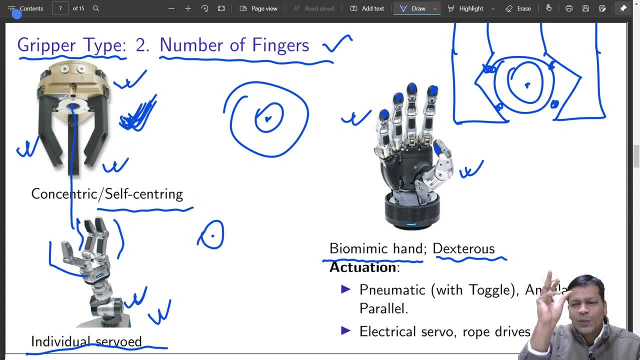 hold, It can rotate something Like a tennis ball. if you hold, you can rotate using just your fingers. Those manoeuvrability is there, definitely, but they are hugely expensive. So until and unless you need something. So this is the main thing. 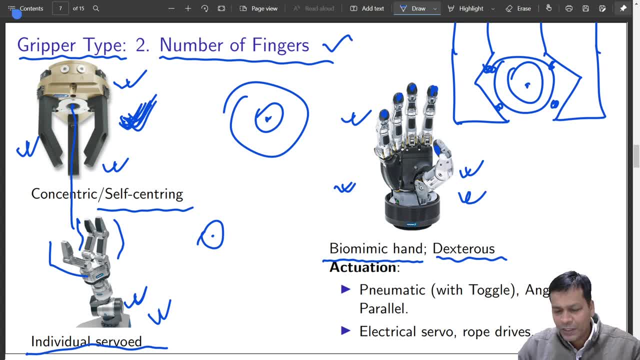 If you need something which requires that thing, you should not go for it. Everything comes at a cost and complexity also. So that is the reason these type of these grippers, they are very, very application specific, So pneumatic finger with a toggle, angular or a parallel, so they can have multiple types. 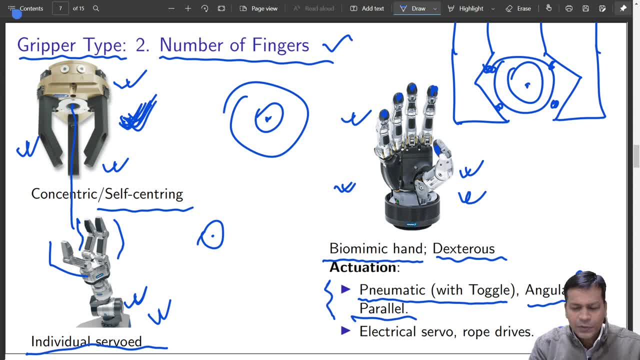 of actuators for these also. So that is the reason You can even have toggle arrangement in this also. even in case of three fingers, each of them can be a toggle arrangement. It can be angular, It can move parallel. also Over here these were moving in parallel. 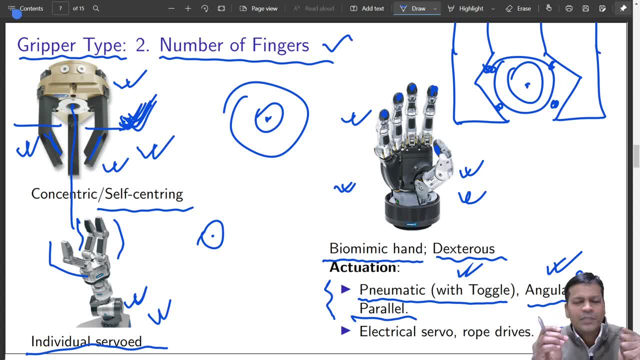 This was additionally helping it to envelope something that it grabs, So it can even move in an angular way. Electrical servo or rope drive servo: Ok, So in case of multiple finger gripper, they are run by ropes. They are not directly. you do not have motor here, motor here, motor everywhere. 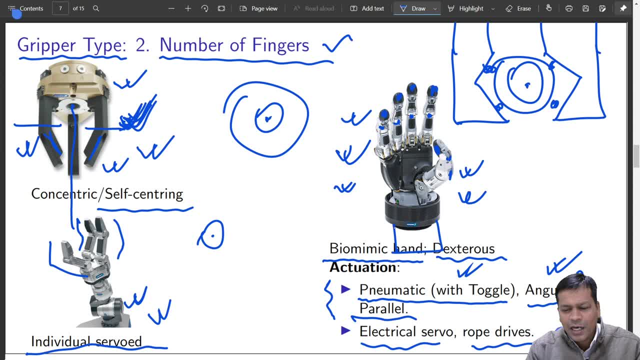 Rather, all the motors are somewhere in its arm and it drives using a rope that goes to all of them. That is the normal way these fingers are made, Because it is very difficult to attach an actuator- multiple actuator- at these locations, So there are various ways. 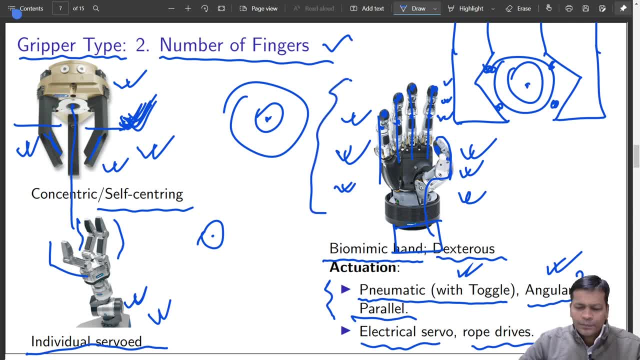 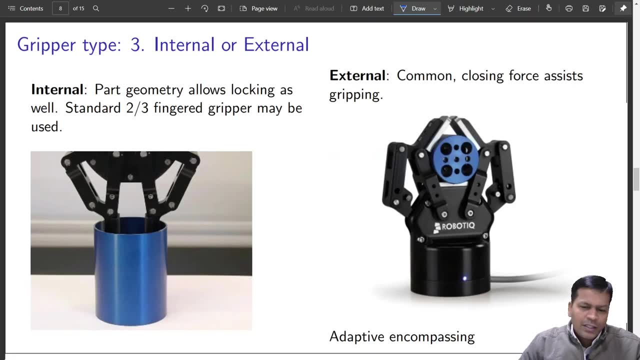 Ok, So this mechanism, how it works. So normally they have rope drives for bio-mimic arms, Even for this one, But this one is direct drive using electrical servo, So that is based on number of fingers. There are some other types of gripper which can be classified based on internal or external. 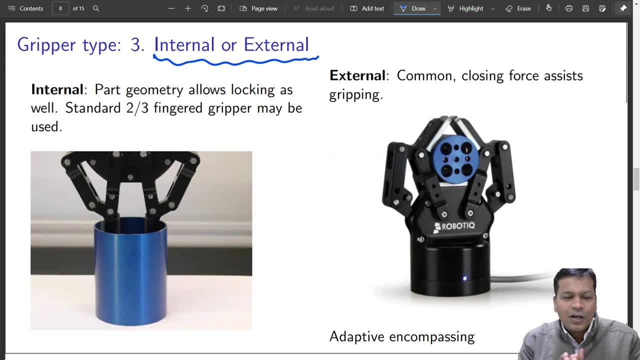 gripper. You can either hold it from outside or, if at all you have to pick up something, you can hold it from inside also. For example, let us say you have a pressure cooker right that has to be picked up. Holding it from the external side, rather, what will happen? basically, it is very big. 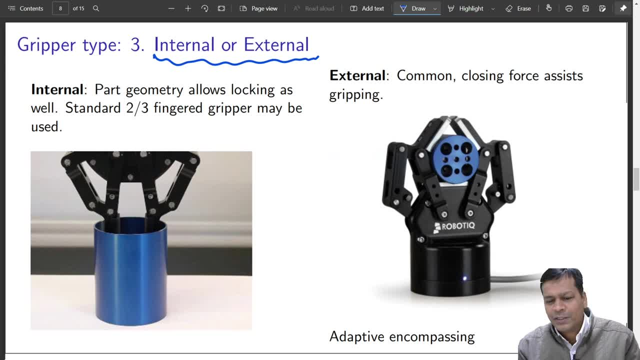 inside. You have to have a huge opening and closing arrangement. Ok, You can hold it from inside, and more so, external surface of a cooker or pressure cooker is smooth. Ok, It can slip off. You can hold it from here. So it is better, or not? 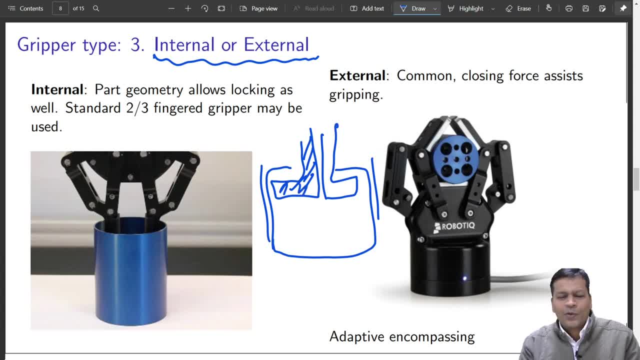 Right, Your finger goes from inside and it stretches out right the way this is shown, So it there is very less probability that it will slip off. rather, it is getting locked from inside of it, right, or this is. this is internal grasping, ok part, or the geometry. 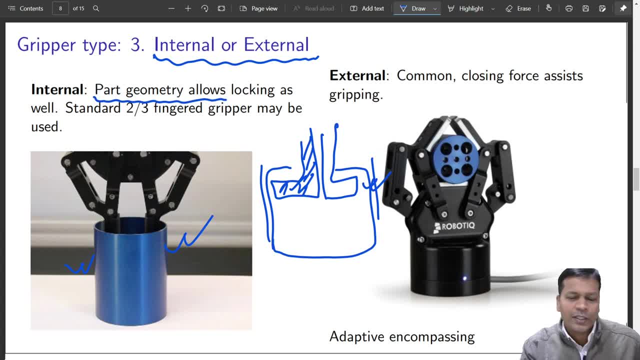 the part itself has a geometry that allows locking, Then only this is possible. It can be a two or a three finger, both are equally good for this. ok. or an external grasp ok, which is commonly used. closing force assists in gripping. 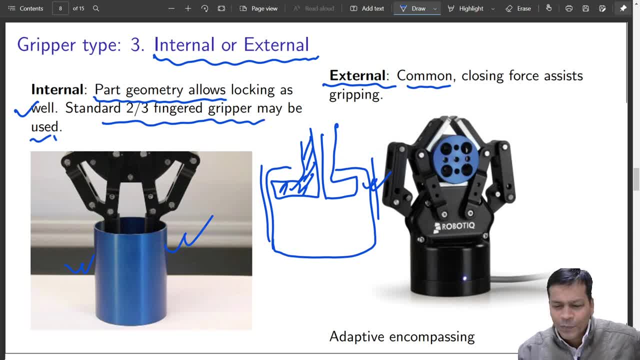 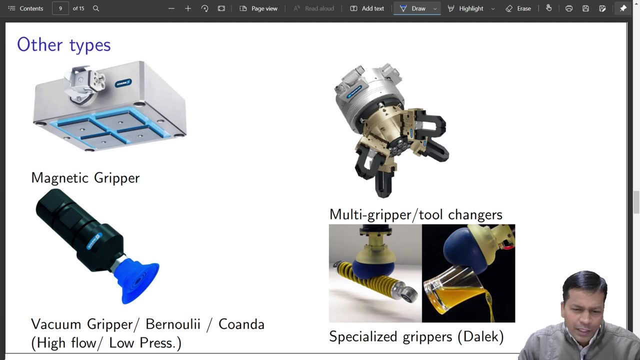 Higher is the closing force, higher is the gripping? ok, But you may require something which is enveloping this- It is known as encompassing- ok, Encompass, It holds from all around, ok. Yes, And there are many other types of gripper- ok. 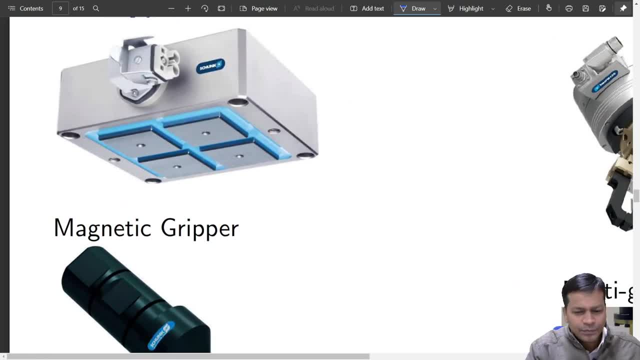 One of them, very popular one, is magnetic gripper. You have huge electromagnets here. ok, like a garbage segregator, where you just want a metallic parts, ferrous part, to depict out from your bin, You can use this type of gripper. 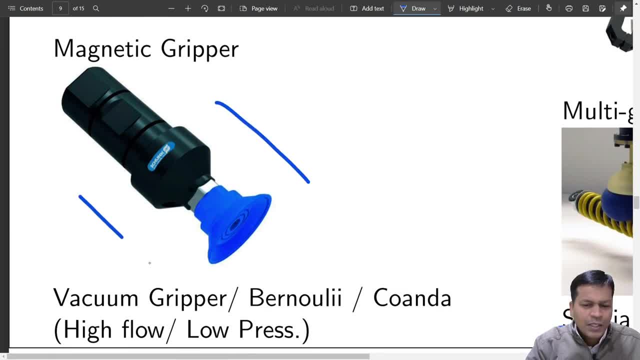 These are electromagnets. You have vacuum gripper. This is not just a type of gripper. you have a wide variety of vacuum gripper. ok, You can have four suction cup, three suction cup like a glass surface, if you want to. 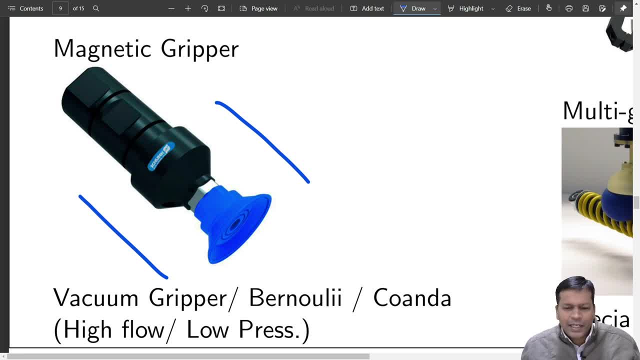 hold a glass ok, a panel, something like that, then these are very, very useful. ok, You can have multiple vacuum suction cup. you can pick it up and you can place it two other place. ok, These are normally rubber faces, ok. 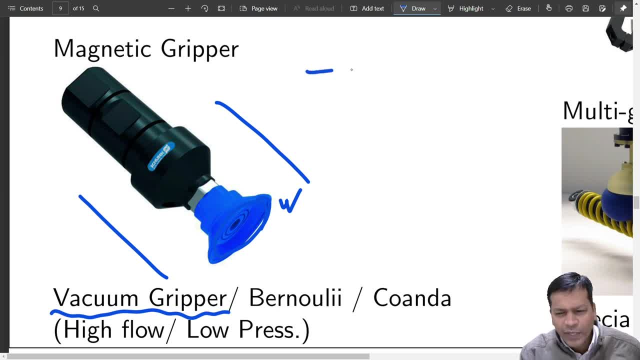 Vacuum. Vacuum can be straight away vacuum, or sometimes they are generated using Bernoulli's principle. What is that? What is that? See, you have a venturi like this. ok, So if you flow in compressed air and vent out from here, ok, you vent it out this. 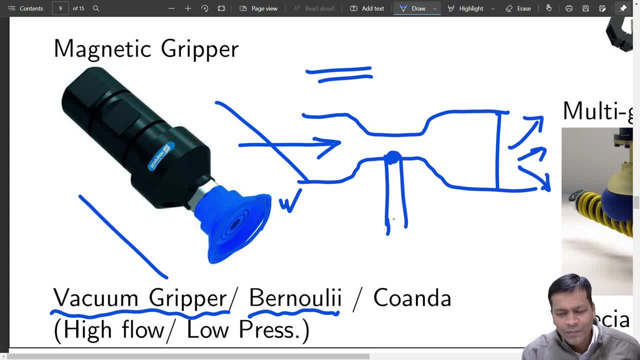 if you have a hole over here, what this will have? It will try to suck in air from this, is it not Ok? So there is a low pressure which is created here because of high velocity, if you remember? So you can have a gripper cup, suction cup, over here, ok, 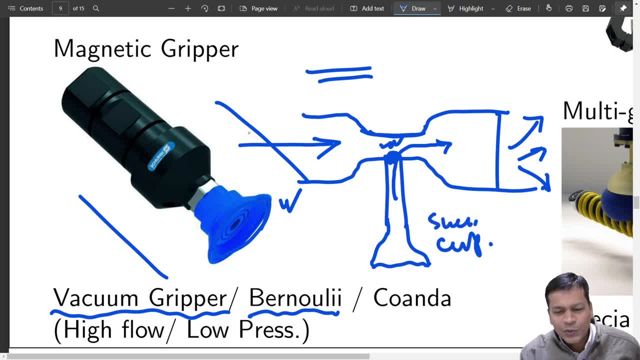 This is a suction cup. ok, So you just create a small vacuum using a flowing fluid. this is using compressed air. you are creating a small vacuum. This is also doable, So a compressed air line. you do not need to have a big vacuum. 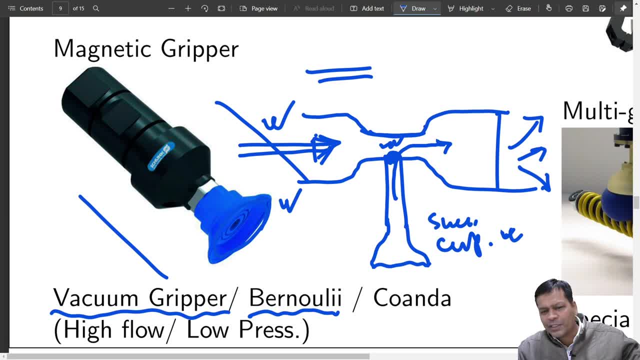 You can have a small vacuum. This is also doable. There is a dedicated compressor for that. rather, you can create vacuum using small vacuum. These vacuums are not very strong, but enough to hold at least small buns chocolates. 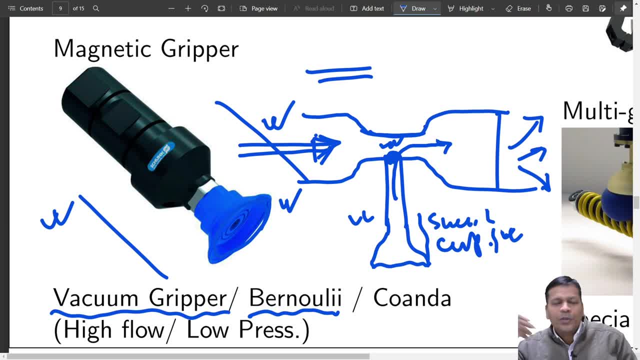 This is very widely used in handling food products. vacuum ok, very widely used Because they do not do any harm to the object that it is holding and most of the food products they are packed with. vacuum ok, So this is a vacuum. 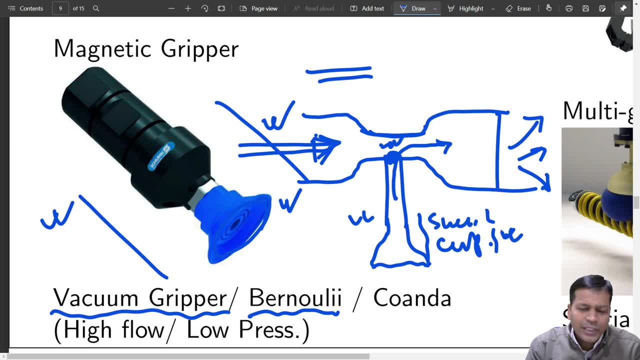 This is a vacuum, So it is packed in polythene, So it does not suck in anything. ok, And polythene products can be easily picked up from this. So wafers, bread packets, any pickle packet, anything. 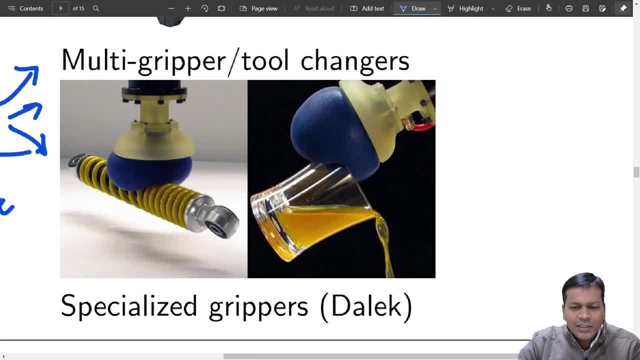 And there are some specialised gripper. This is one of them, if you can see this. So multi gripper, tool changers- Tool changers is a different thing that I will show you. So what this is, So what this is actually. 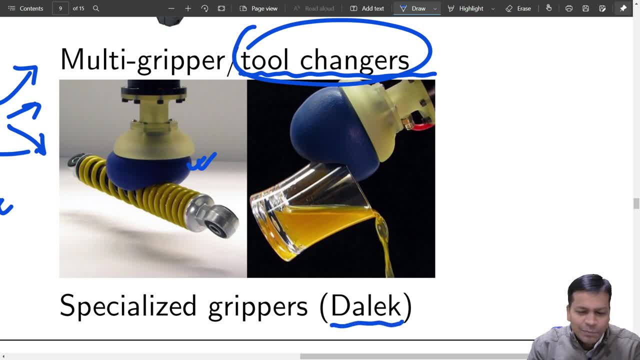 This is a Dalek arm Dalek gripper, a specialised gripper which can take any shape that it comes in contact with. How is it possible? Have you seen a bean bag? You have seen a bean bag. It is just like that. 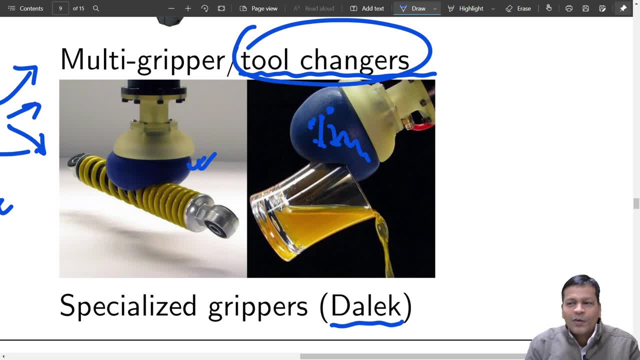 It is just like that. You have beans like a thing inside. Okay, So what you do? You press your gripper. you press your gripper on top of surface that you want to hold and then you pull out air from inside. 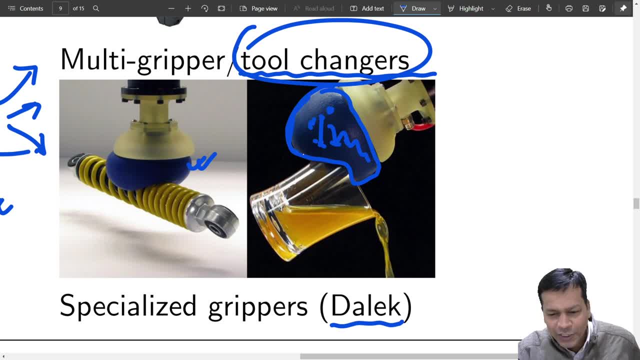 What will happen? The shape of this bean bag will freeze, freeze to the shape of object that it is holding. Or sometimes you have iron, ferrous particles inside. And what you do? As soon as it comes in contact with the object, it will freeze. 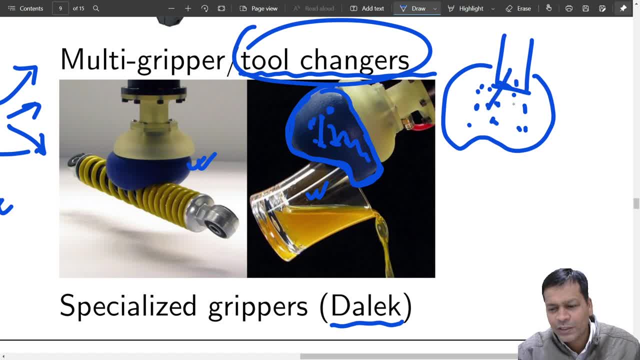 You apply an electromagnetic field to this, okay, All the ferrous particles will get frozen there then, and there It becomes like a solid and it holds something, So you can take the shape of an object, freeze it and pick it up. 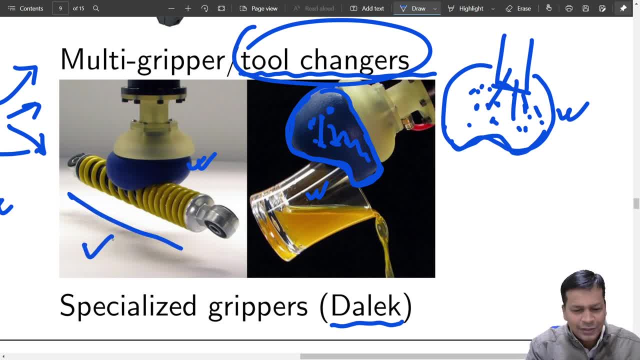 So that way you can do hold like this object. You cannot apply a vacuum gripper here. You cannot apply a two-fingered gripper. You need to have a multiple type of gripper here. So rather use this type of thing. 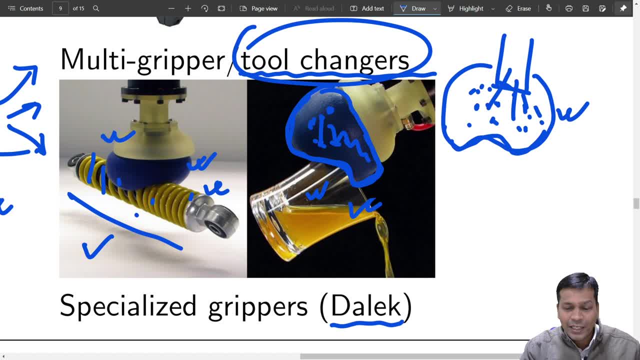 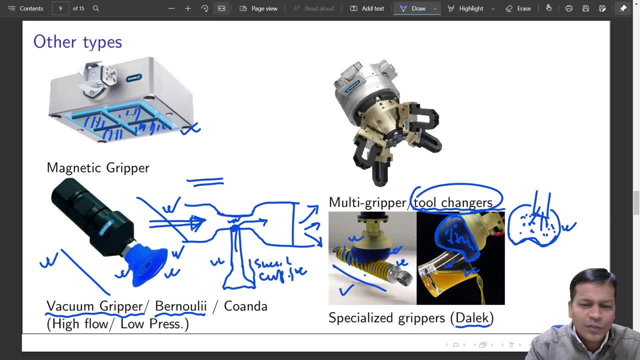 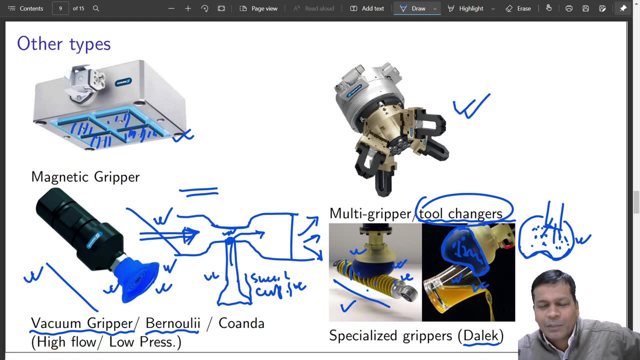 But they are very expensive too. okay, You can hold glass. They are compliant. also, You can hold fragile objects very easily, okay, So that is a very, very special type of gripper, okay. So, yes, you have something which is called a tool changer or a multiple gripper. 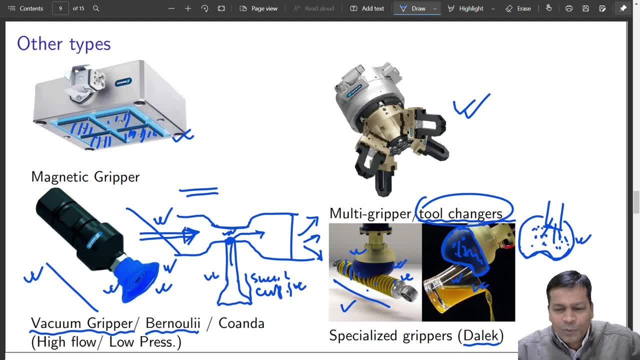 Instead of having a unique, one single type of gripper at the robot end. If your robot has to handle multiple scoops of different sizes and put it to the assembly line, you can have a type of gripper here, you can have a gripper here, here, here and. 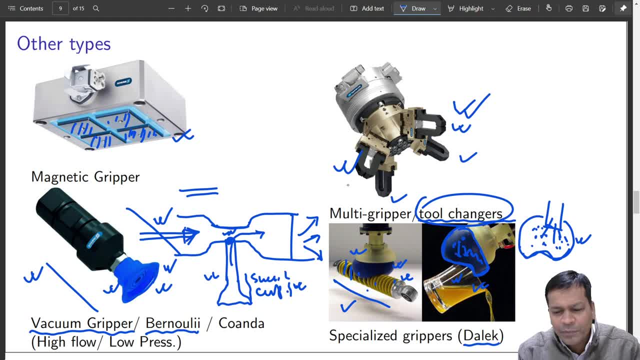 it can rotate, rotate, rotate At a time. you can use one of them. So you have one gripper two, gripper three. So based on that, you can. it is like our Devi. no, that you have seen. 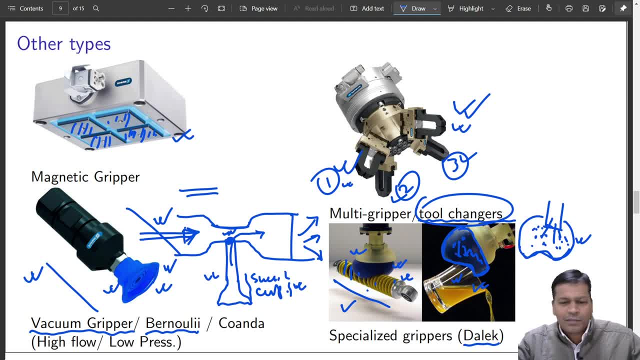 Ten hands. You can Ek mein talwar hai, Ek mein yeh hai Ek mein hai. You can have hold multiple things So same way. It is like goddess no. So they can hold anything. So it has four different types of gripper and, depending on the use, it can rotate and 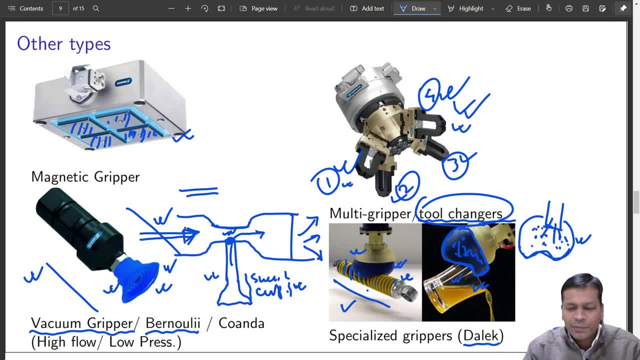 it can hold using one of them, Or you can have something which is known as a tool changer. It is not just a gripper, It is an interface between robot arm, and maybe you have a type of gripper which is here. Okay, 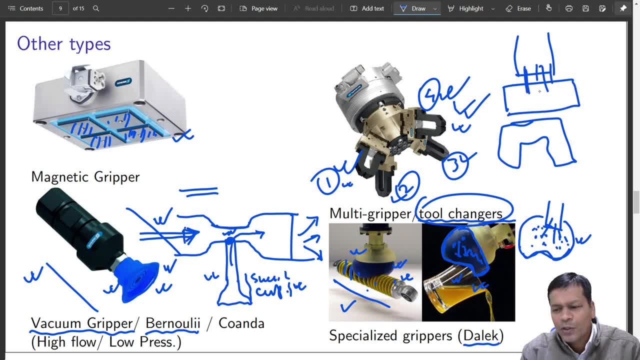 So you have an interface which is fitted with the robot. And what this does? this tool changer can pick up any of the gripper of its kind which is required, So it sees the object. Then you take the robot to the type of tool which it needs to handle that kind of object. 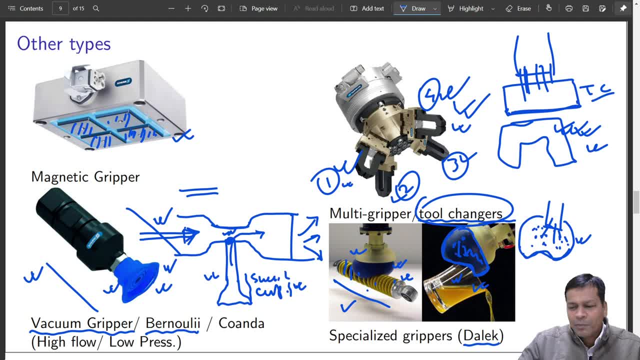 It picks up that tool, Does the job, Places the tool back in its place, Picks up another tool, Does some other job, And again it keeps on doing that. Okay, Like the way you can do- sometimes you can hold a hammer, sometimes you can hold a chisel. 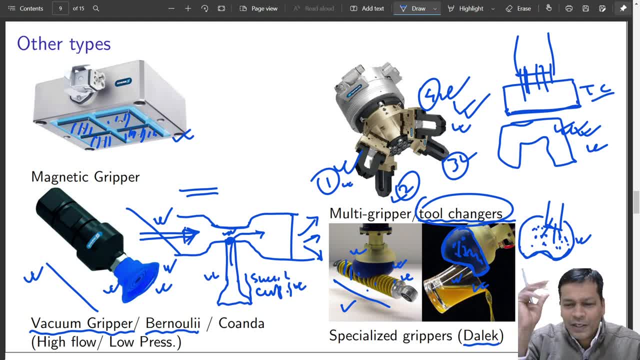 So you can hold multiple things using your gripper, your hand. Okay, This tool changer does type of this type of job. So this is not a gripper, This is a tool changer, So you can have an interface that lets you have multiple things. 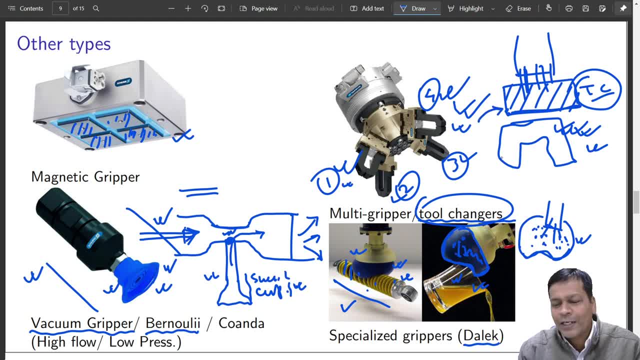 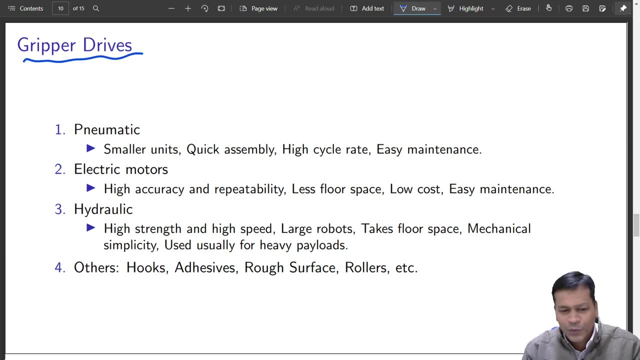 So this is not a gripper, This is a tool changer. This is a tool changer that lets you handle multiple type of gripper at its end, Okay. So this is all about gripper so far. Okay, Now let us see what all types of drives that can go in. 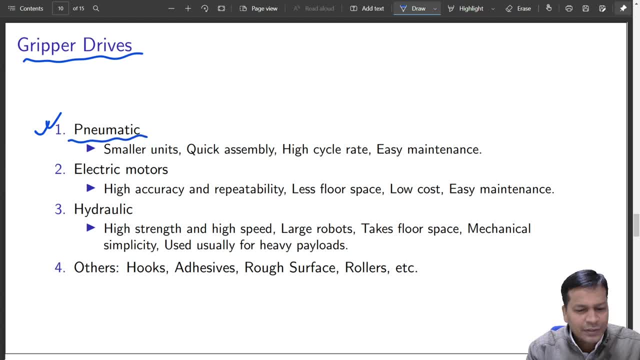 You know very well, I would talk about pneumatic that can hold things in small units. Quick assembly, because they are very, very fast and cycle rate is very fast as well. You can quickly open and close that type of drive. Okay. Easy maintenance because you know there are very, very less parts which are there. 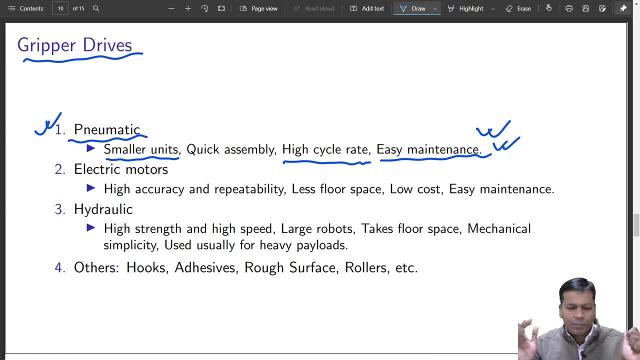 So they are very, very reliable. So that is the reason they are naturally compliant also. You know, with pneumatics they are naturally compliant, So they are safe for the environment also. So that is the reason. this is the one which finds its use to the maximum in the industry. 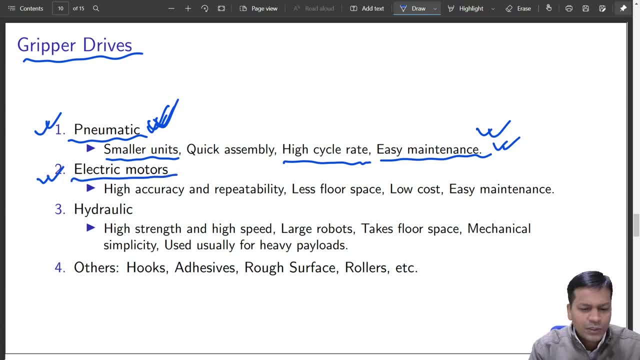 Other very broad category. they use electric motors. They have high accuracy. You hardly need very accurate grippers, Okay, Because your object sizes they vary, Until unless you are handling something like a PCB or a IC chip. Okay, So in those cases you prefer using these. 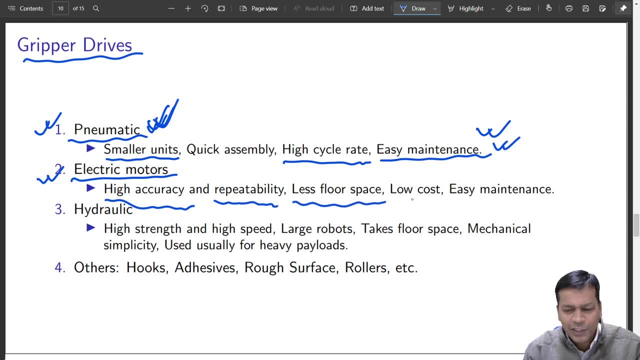 They are very, very repeatable. Less floor space is required because electric motors they act then and there. They do not need a compressor and an air portal and those things. They are low cost, easy maintenance as well, Not as easy as this one. 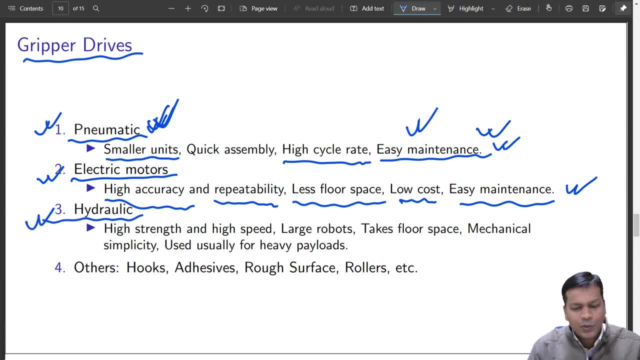 Hydraulic. that is required at an extreme case. you know when you need to handle huge amount of load. You want a huge gripping force to handle something Right. It takes a floor space, large floor space. Mechanical simplicity is there, definitely Usually used for heavy payloads. 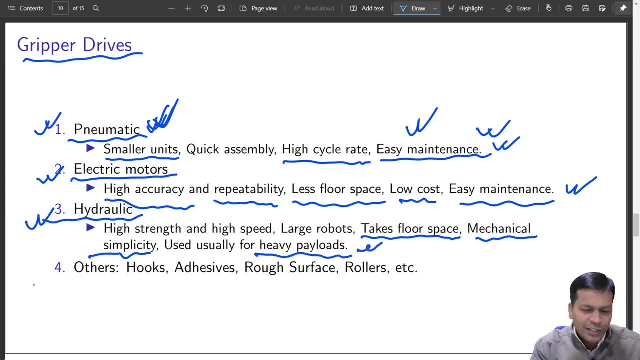 Okay. Others are non-conventional. ones are: although they are present, They are hooks. Even hooks are there. They have no, nothing like a crane. No, You can just have a hook. You can just have a hook, Entangle it. 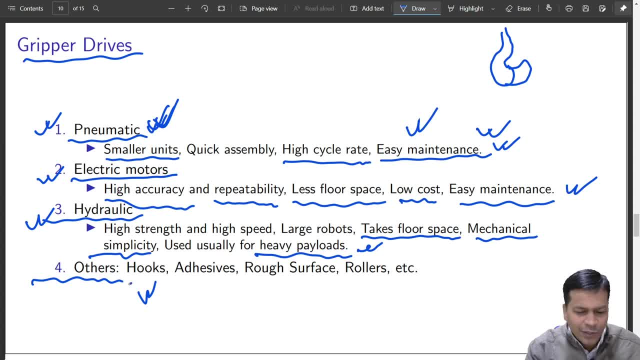 Right, You pick it up, place it somewhere. So that is a hook. You can even have an adhesive- Adhesive that just glues it, put it somewhere. But how to unhook that? in that case, Okay, You can swipe it out. 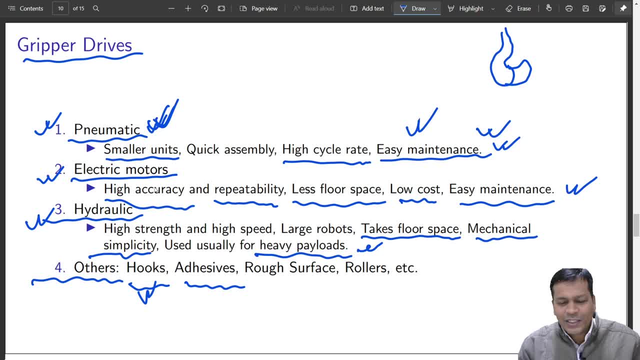 Okay, You can swipe something on the surface and you can take out Right Adhesive Rough surface is also a type of gripper You can in order to drag something. if your surface is rough, you can simply drag something Right. 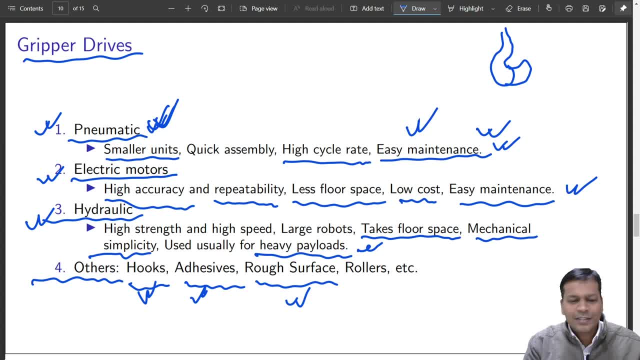 You do not have any moving part in this case. Right, You want to remove something from the conveyor belt? You do not have to pick it up and place it, You just push it Right. This also is an end effector. You can even have a roller for that reason. 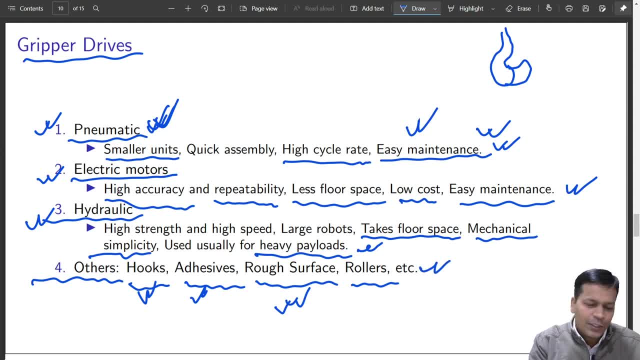 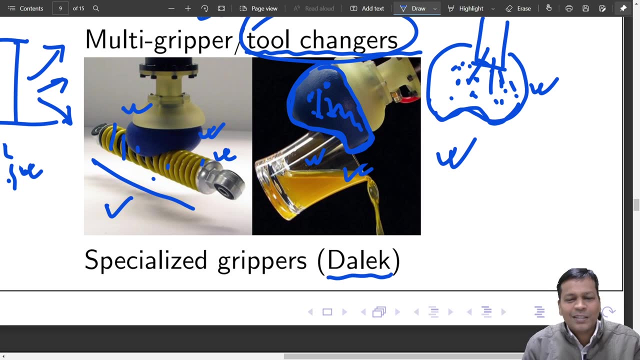 Okay. So these are some non-conventional way you can think of. Do not stick your brain to these type of gripper Gripper. Somebody must have discovered this. Once you can think non-conventional, you can think something like this: 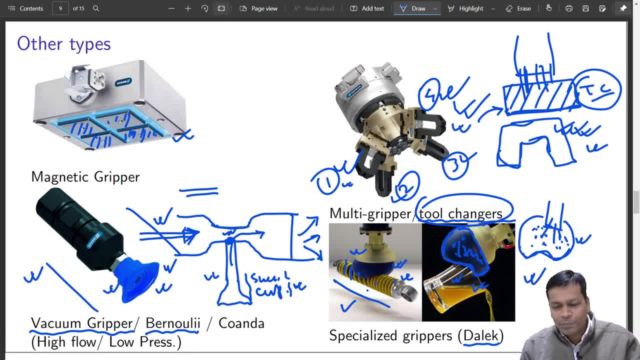 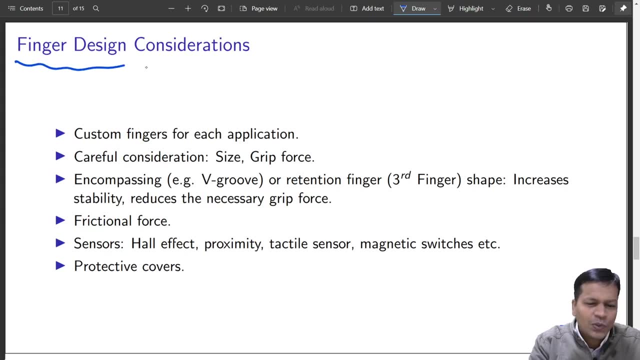 Like a bean bag. No, So this is something out of the box you can think. Do not stick to something that is taught in this class Or your knowledge only. Okay, Yes, Just a second. So, yes, there are many other considerations that you should look for while selecting a. 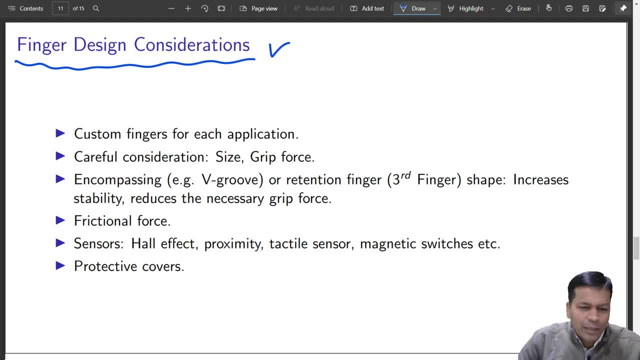 gripper, or selecting a gripper for a particular application, or even when you are designing a gripper. That is quite natural. Yes, You do design a gripper also, if at all you need it in order to go little more inexpensive way of doing something. 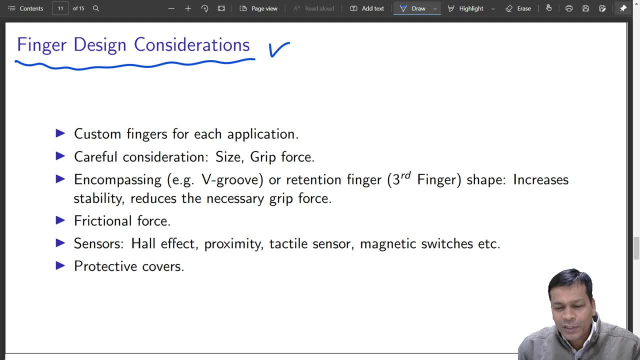 Right. Like in case of our robotics club, students club, they do robotic competitions also. In those cases they do design their own gripper, not just gripper, SI Baha members, they even designed a whole of the car to do that competition. 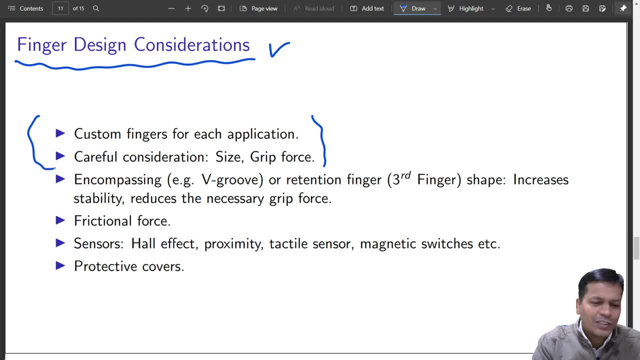 Right, So same way, they can think of that, because they have limited resources, money and everything, You can always have some your own regards out of it. Okay, So custom fingers for each application. You know now, each and every gripper that we have seen so far is very, very customized. 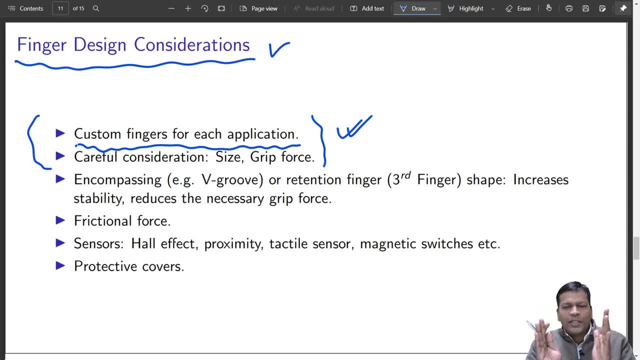 for a given application. Even a parallel finger surface of that can have a rubber pad. That also is a type of customization. Right, You can have a sticky nature, You can have a slippery thing, You can have a curved shape or a wedge, whatever. 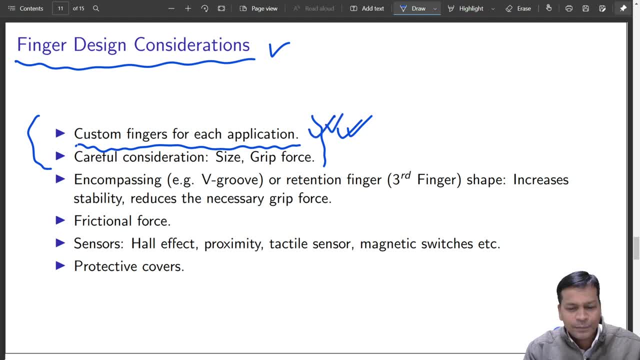 So each finger can be customized Right. So you know now every application you have to customize your finger. Careful consideration on the size. You know how much is the travel of your finger. If you know this can travel by 5 mm only and you have to hold a cylinder which is of regular 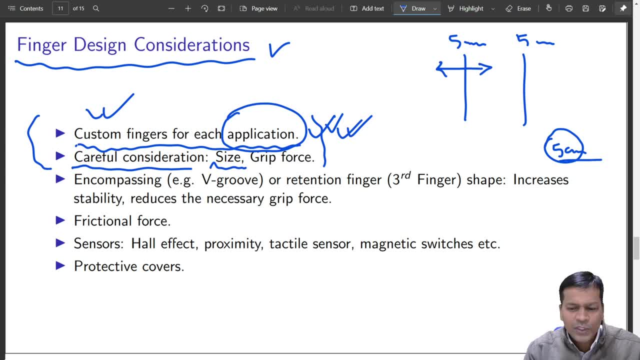 size of 5 cm. so how will you do it? You can attach a finger on top of this, which is normally at a gap of. you can attach something on top of this so that it is when open, it is about 5.2 cm and when it closes it is. 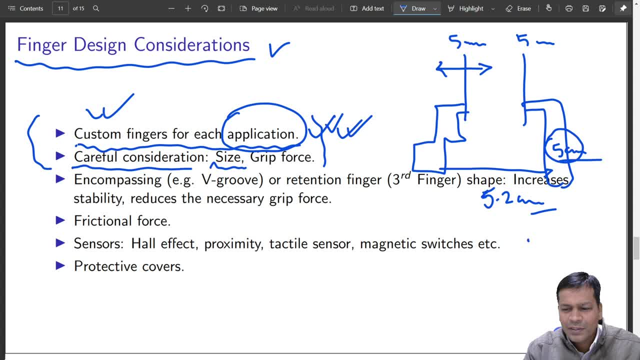 less than 5 cm, Right. So in that case, even with 5 mm opening and closing travel distance of these two fingers, you can hold something as big as 5 cm, even larger. You just need to know how much is the travel of each finger that you can make. 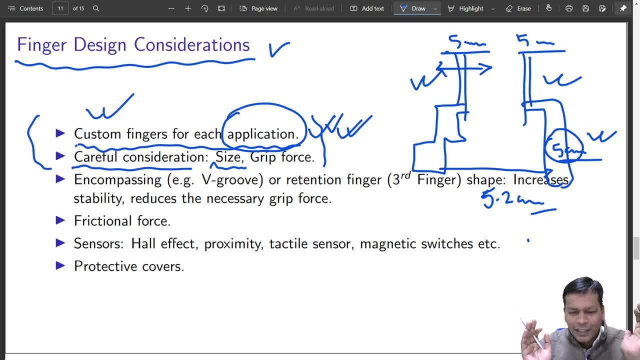 Is it not So? you should understand the application size of something that you want to handle and the gripping force that you desire. Why? Because you know, once you pick it up, your robot is going to move. So either you can have an enveloping grasp or a firm grasp. 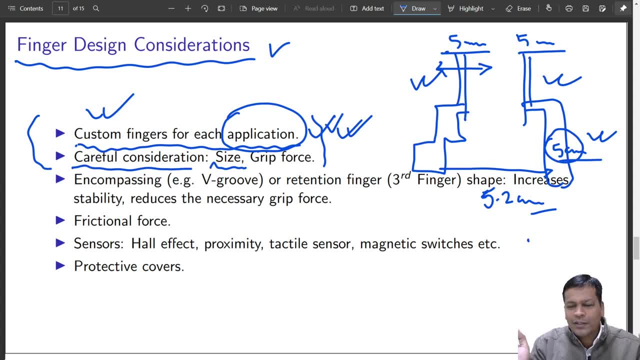 So that it does not fly off from your finger while the robot is in motion. That is very, very unsafe, Right? So normally we do, we do make wedges, we do make circular holes inside. Okay, In the gripper you make this type of surfaces so that you can hold something which is cylindrical. 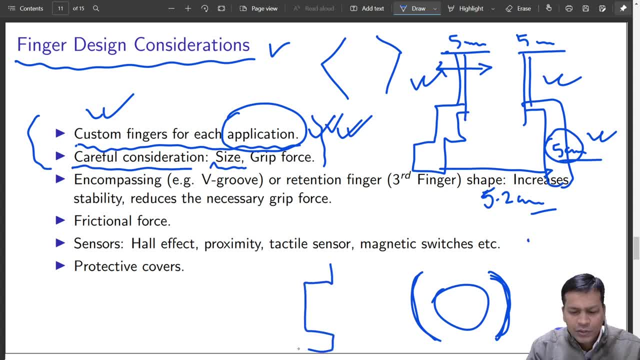 or maybe you can have a rectangular slot Right If you want to hold something which is rectangular Right. So the gripping force is very, very important. Shape and size of the object that you want to handle is also very important. So you have seen, you can have an M-COP passing grasp using V-group. 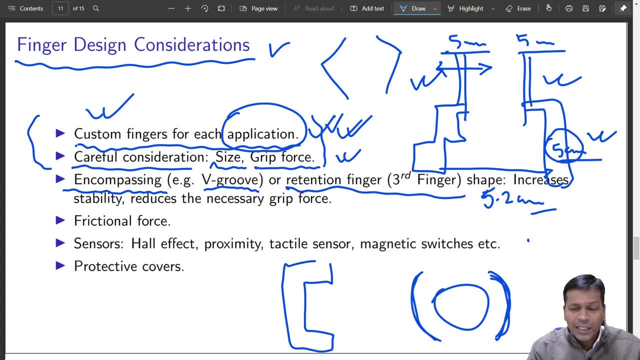 A retention finger, a third finger which may be a dummy also, which may be a dummy also. You have just two fingers, but you can have a dummy tool, support from both the sides If you feel that it can fly off from the other two sides. 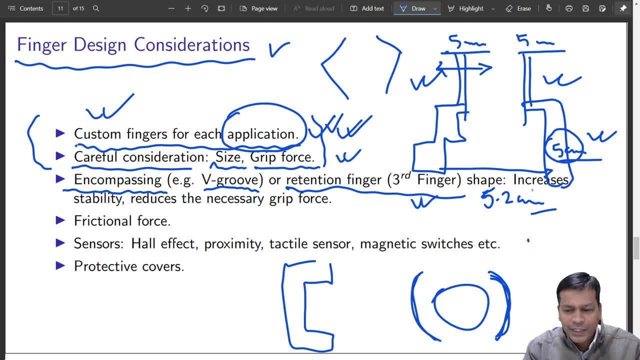 Right, You can have that dummy arrangement that increases the stability and reduces the necessity of gripping force. Friction force in this surface is also very, very important. Right, You can have sensor whether your gripper has closed. Okay, You have commanded your gripper to close, but whether it has closed or not, you should. 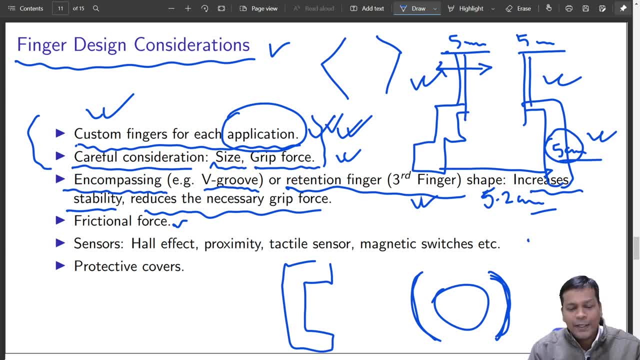 have a close feedback of that. In order to do that, you have what You have: hall effect sensor, proximity sensor. Sometimes you have a load cell. If you have gripped something and you have started picking it up, definitely you will see some load changes. 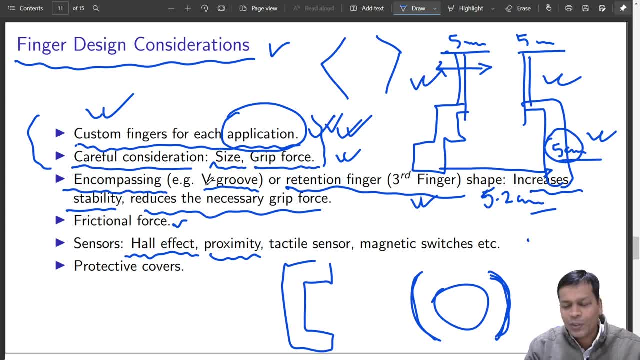 Using that load cell also, you can come to know: yes, now I am holding something. I am not returning empty handed, Right? So tactile sensors are there in order to detect some slip. Magnetic switches are there. Sometimes you have protective covers also. 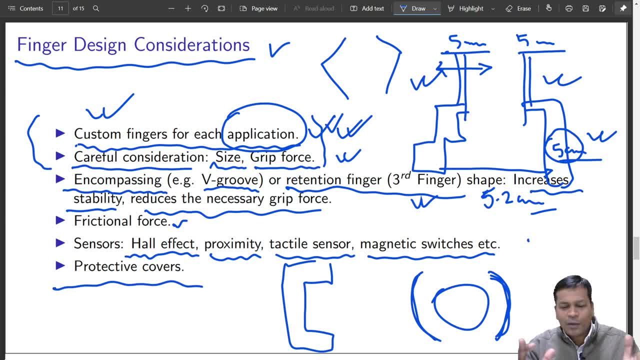 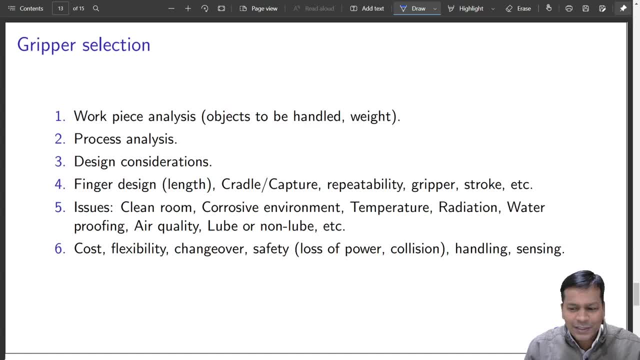 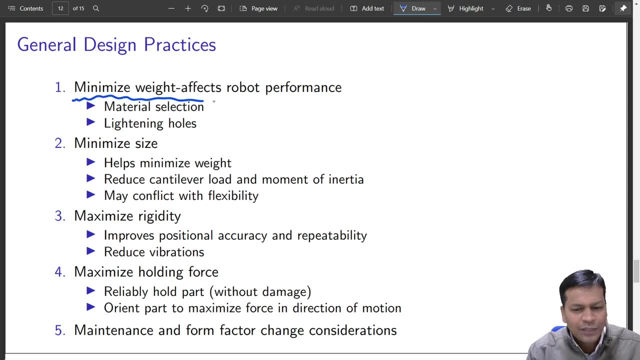 As I have said, you can have protective covers so that your object doesn't fly off once you have hold it Right. So general design practice is there. Okay, What it says, as just now I have discussed. so you have to minimize the weight effect. 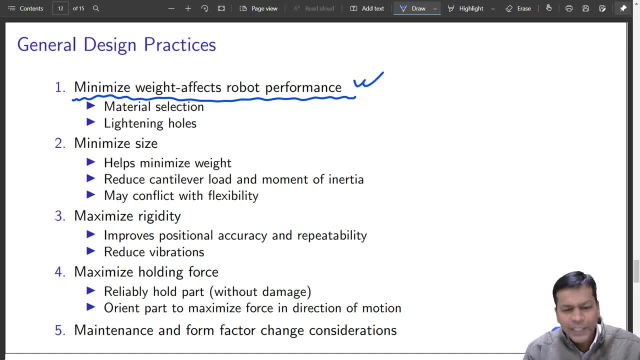 on the robot performance Right Based on that, your finger, your whole of the gripper is part of the patient. Let us say your robot can handle 5 kg of payload and your gripper itself is of 3 kg. So how much load that additional it can carry. 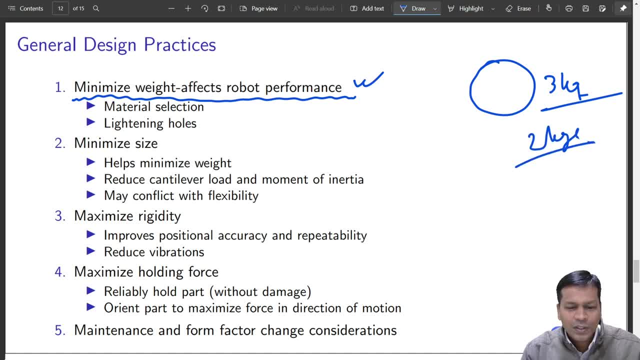 2 kg only. Right, So your gripper itself should be of lighter materials. Right, So that material selection is very, very important. If required your finger, If it doesn't require too much of, If required too much of strength, you can drill holes on that. 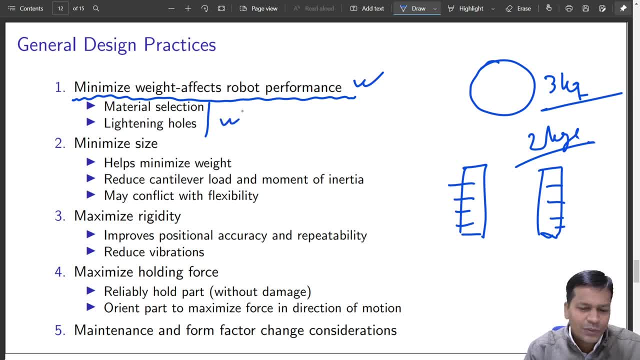 Right So as to make it lighter. So that is something which is to be done: Minimize the size Right, Which helps minimizing the weight that you have seen just now. Reduces cantilever load. If you can handle something with a small finger, why to hold it with a tongue which is very 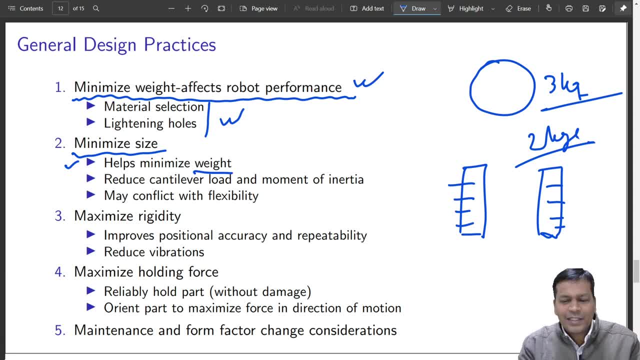 long Right. So unnecessarily designing a finger which is very, very long Will unnecessarily create cantilever load on these actuators Right. So you have to design this so as to have minimum cantilever effect. Moment of inertia is also increased if you change the length of your gripper fingers. 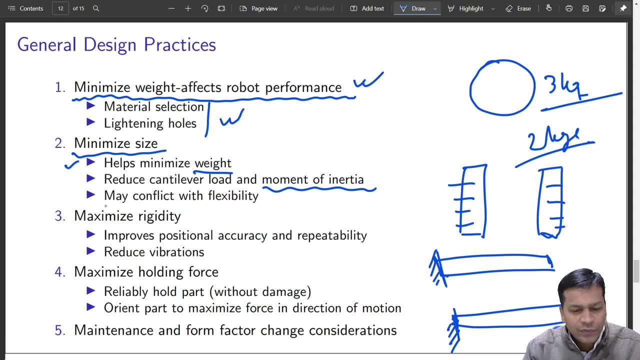 Right, But yes, they may conflict with the flexibility. Okay, If you reduce the size, you are less flexible, Right. So if you need some flexibility, some compliance in your design, you may have a longer finger also. Yes, Maximize the rigidity. 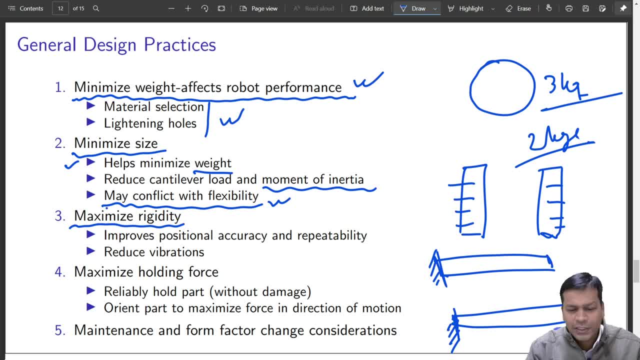 Again, reducing the length will maximize the rigidity of the finger- Okay. It improves the positional accuracy and repeatability of this finger Every time it closes it leaves there. Okay, It also reduces any vibration and its after effects- Right. 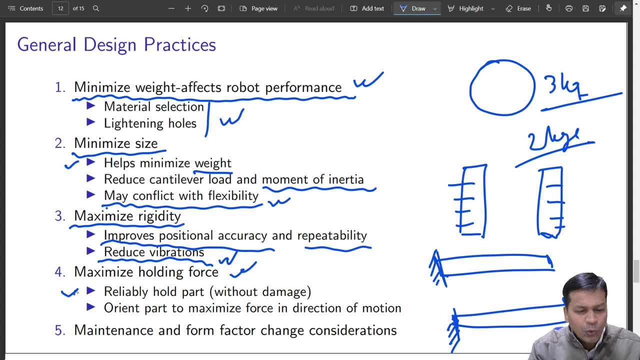 Maximize the holding force. Reliability to hold. This is very, very important, But without creating any damage to the object. Right Holding force has to be optimized. It should not be too much. also, Orient part to maximize force in the direction of motion. 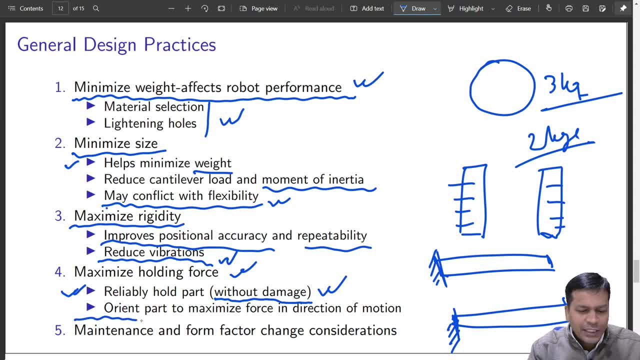 Right, This is something which is to be taken care of by the programmer also. Okay, You have to orient this part so as to maximize the force. Right, Let us say you have a gripper which is this long You have to hold an object. 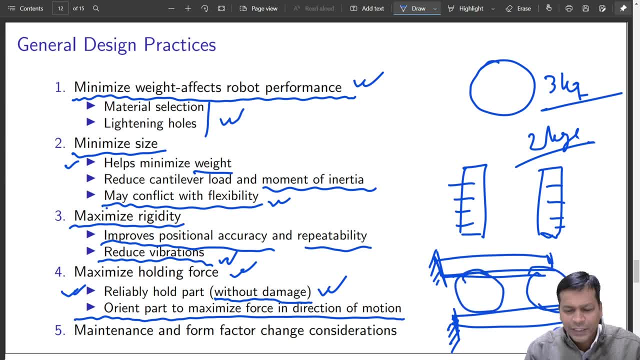 So you can prefer it holding here. You can prefer it holding it here every time it holds, Okay. So, depending on the size of the object and the situation, you can plan, you can program accordingly so as to have maximum gripping force. This is the place where, with the same amount of torque, you can have better force. 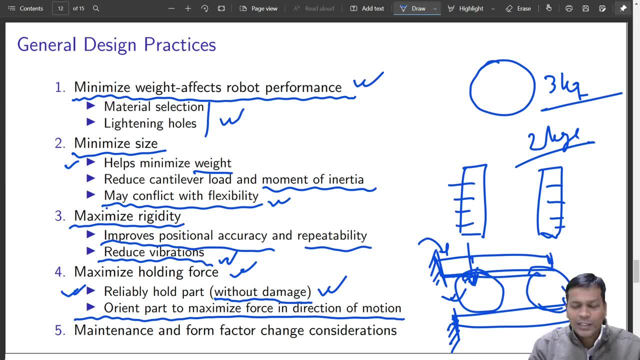 Right. So this is something which is to be noted for an angular gripper, at least If it is angular gripper with the same torque. you see more force which is getting generated here, less force over here, Is it not? So you have to orient your part. 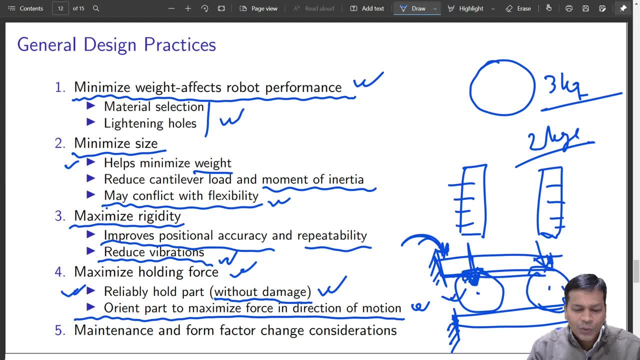 You have to precisely plan your part so as to hold it properly And maintenance and form factor changes. So if at all you can handle with parallel finger, why should you handle with the rotary fingers or angular gripper Right? Unnecessary maintenance will come. 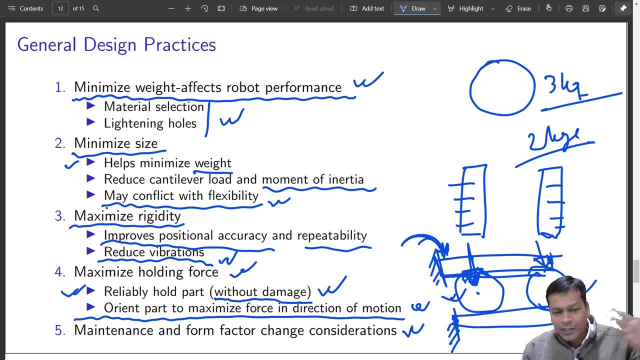 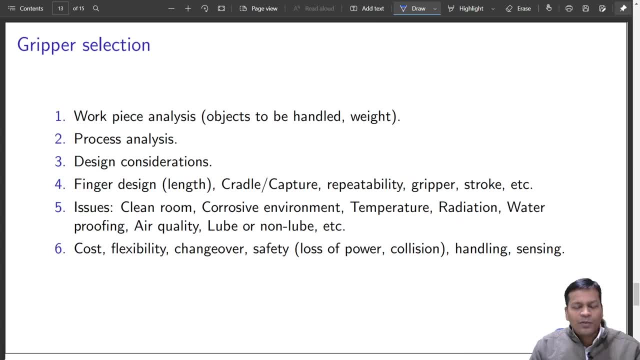 Right. So these are some of the design practices, or even selection. you have to be very, very careful. So what we have done for the design, we have to take care while we do the selection of any particular gripper. So you have to do workpiece analysis. 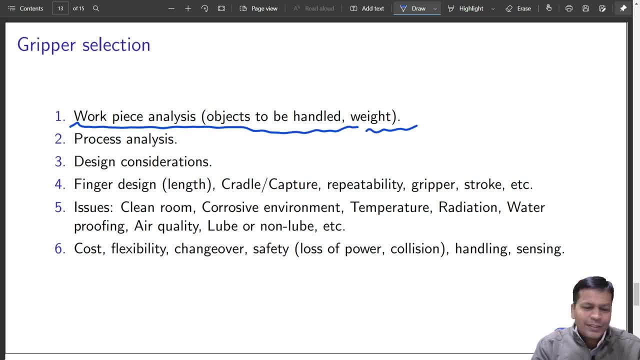 Okay, Object must be handled. What is the weight Process analysis? That means if you have to move with one meter per second, it's quite high of a velocity. If you have to move very, very slow, it is okay. You can hold with minimum amount of force and you can handle that. 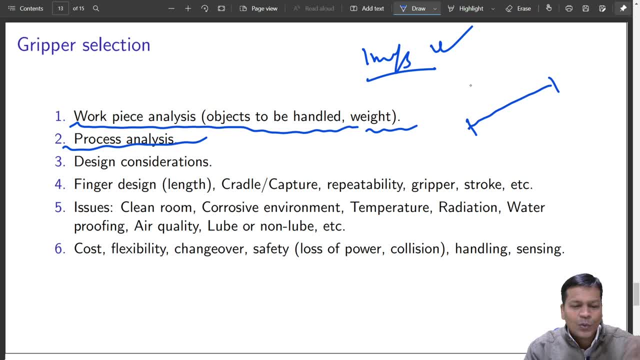 You have to take care of the dynamic effects of load also, So you have to analyze the process Right. Whether you are picking up from a conveyor, putting it to a basket, it is good, But if you are picking it from a conveyor and it is like a knife, you have to cut something. 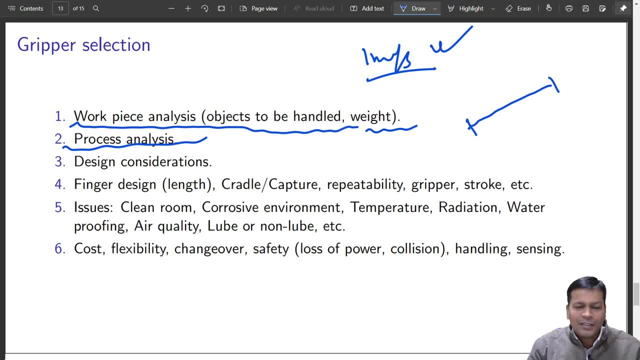 definitely. you have to very, very be careful about its path, your trajectory, your dynamic effects, many other things. Okay, And definitely the design consideration, something that we have learned just now. Okay, Finger design should be like a cradle, or it should capture the object. 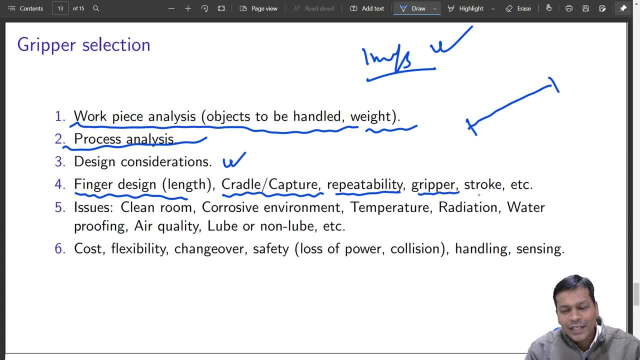 It should be repeatable. Right, It is like a gripper Stroke length and all is to be taken consideration. how much is the stroke length We have just seen with an example, while holding a 5 centimeter object just now? Okay, 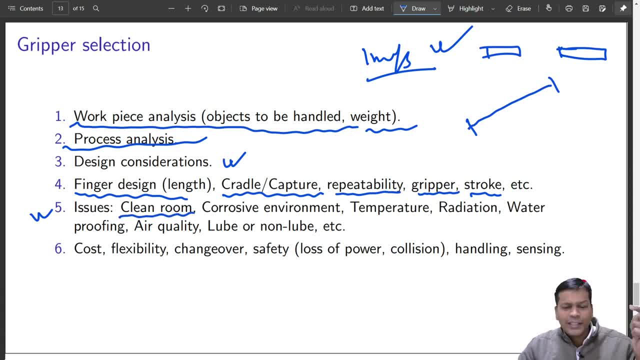 Issues like a clean room. If it is a clean room, what is a clean room? What is a clean room? anyone Clean room is basically a room where you have a limited amount of material. If it is a 100 class clean room, that means 100 particles of 1 microns will be floating. 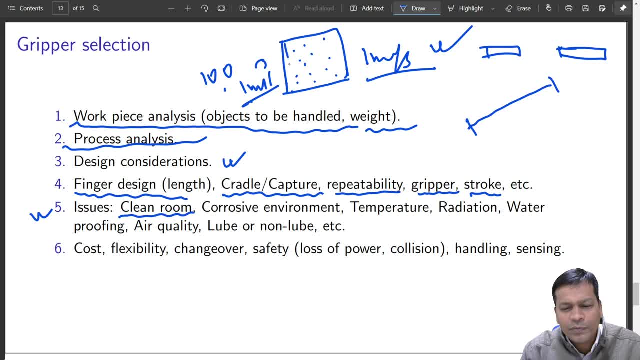 in 1 meter cube- 1 meter cube of air- at that region. So that is a clean room. It is mostly used for IC fabrication and precise electronics manufacturing thing. Okay, So in those cases you have to be very, very careful while choosing a gripper.